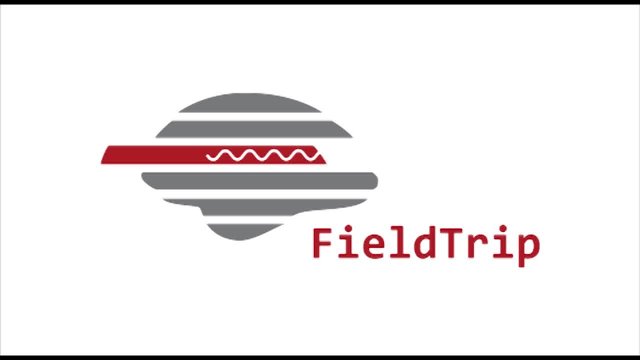 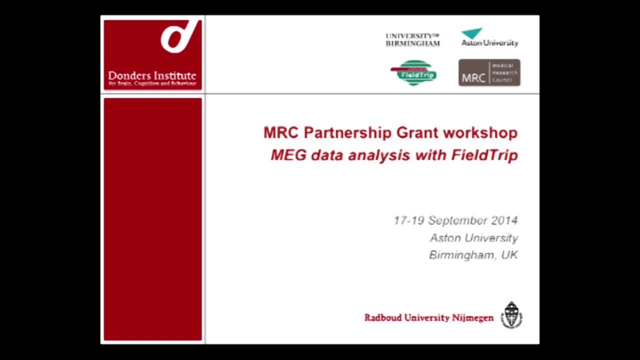 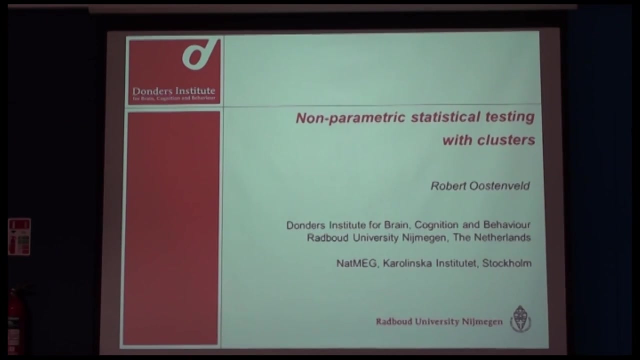 Welcome to a Fieldtrip Toolbox video. You can visit us at fieldtriptoolboxorg. So the plan for this morning is that I'm going to talk you through the statistics lecture. like the method that we're using for doing statistics, and I know that many of you 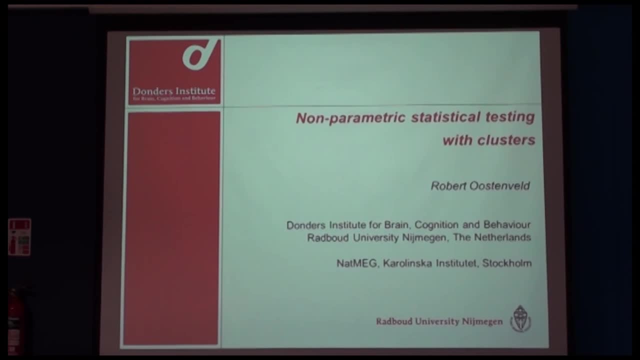 will have already have had statistics in at university, but the way that we're doing statistics is rather MEG specific, or EEG and MEG specific, so that's that's why we want to explain this as well, and it's a it's a method that we started developing, like about. 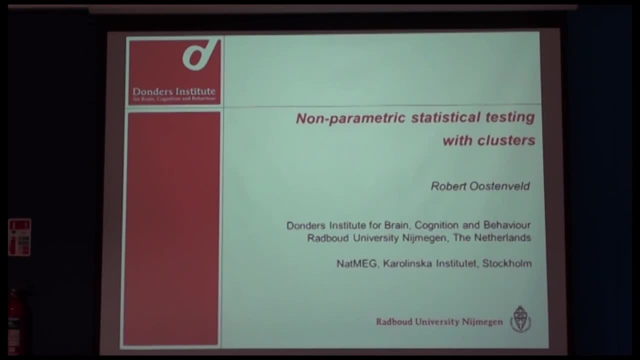 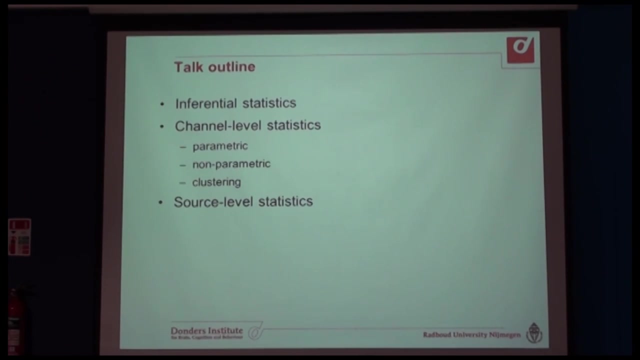 five years ago and and it has picked up quite a lot of attention within the field of MEG, and it's about non-parametrical statistic statistical testing with clusters. The outline of the talk very shortly recapitulates what inferential statistics is about, so I tend to make a 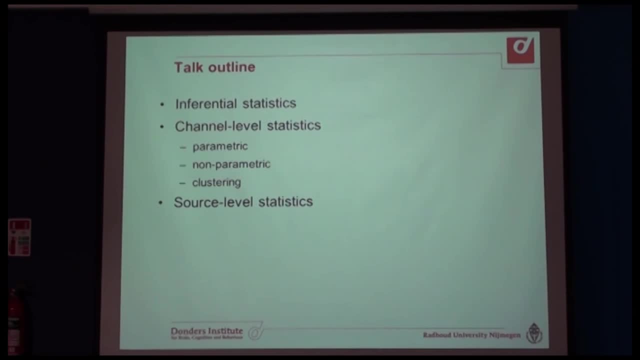 difference between inferential statistics and descriptive statistics, or modeling. Inferential statistics is about making decisions. Then I will spend most of the time explaining the method using channel level data, but towards the end I will go to the source level and I will explain how, how the same mechanisms can be done on the source level, and already yesterday we were talking about how we can use this method to do data analysis. 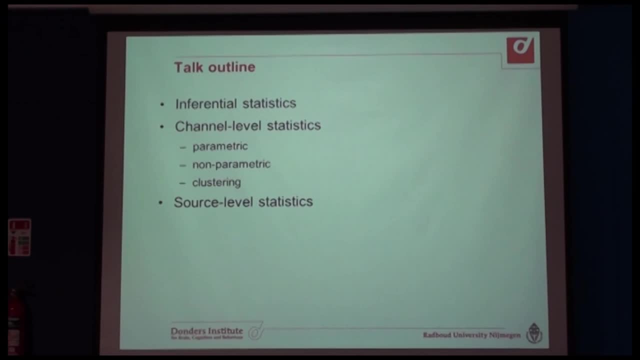 I will go to the source level and I will explain how how the same mechanisms can be done on the source level. we've been mentioned these, these common filters, quite a few times, so I'll again be explaining what the relevance of these, of these common filters are, and and why they also pertain to statistics. 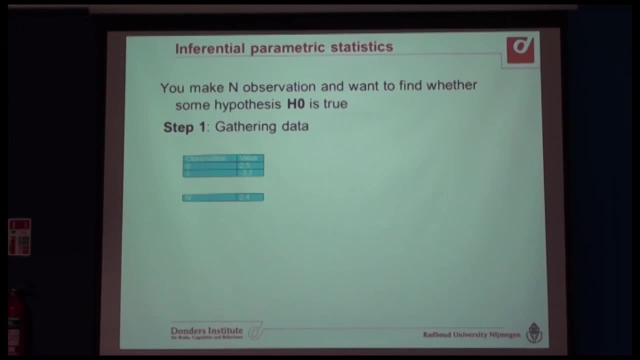 but let's start by inferential statistics. so what we have is we have a, an observation, and we want to find out, basis on the base of that observation, whether some hypothesis holds. actually, this should have been a, an alternative hypothesis. so usually we start with the null hypothesis and we're interested in showing that the alternative hypothesis is the null hypothesis. 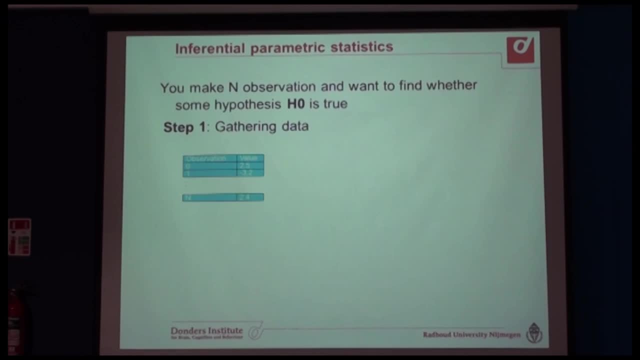 hypothesis holds. So what we do is as: first we make observations and then, given those observations, we look at the distribution of the data that we've observed and given a. Please come on in. I just started, so you only missed the overview. So, given the 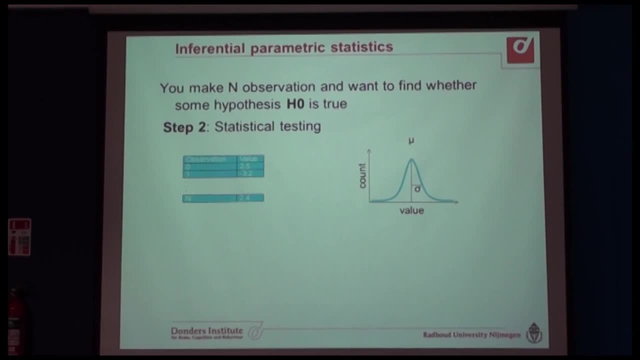 observed data. what we do is we Usually we compute the mean, we compute the variance of the standard deviation and then we determine the probability of this distribution, given a T-score under the null hypothesis, by comparing the mean to the hypothesized mean given the 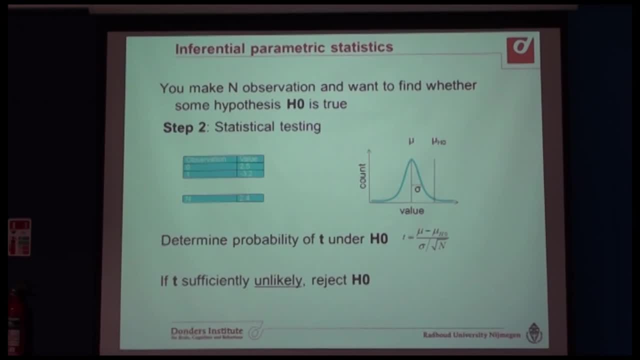 amount of variance that's in the data And if the T-value that we've observed, if that's sufficiently unlikely, then we reject the null hypothesis. It's in favor of the alternative hypothesis. So statistics, inferential statistics, like this is a way of helping you to make informed. 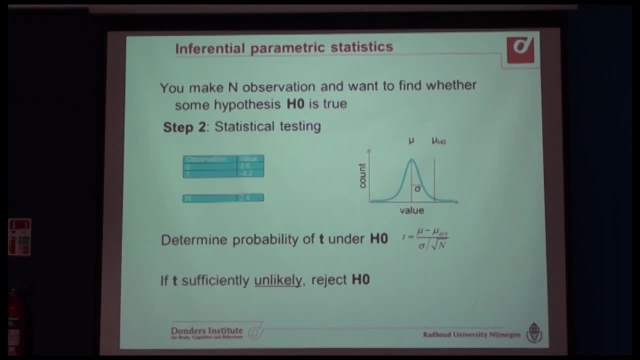 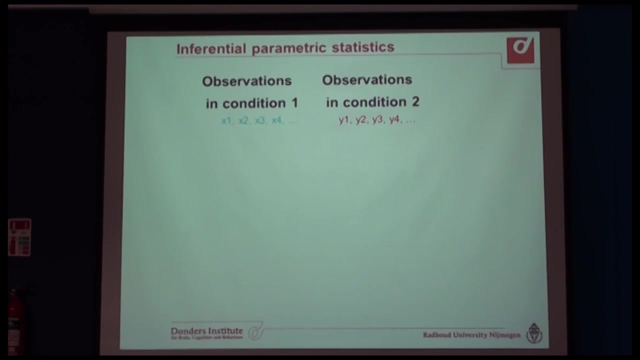 decisions about hypotheses. Curtis Kerr, PhD, UND, MD. Quite often we don't have a single observation. actually, We have an experimental manipulation in which we observe the brain while the subject is engaged in a task, where the subject is engaged in a task with multiple experimental manipulations. 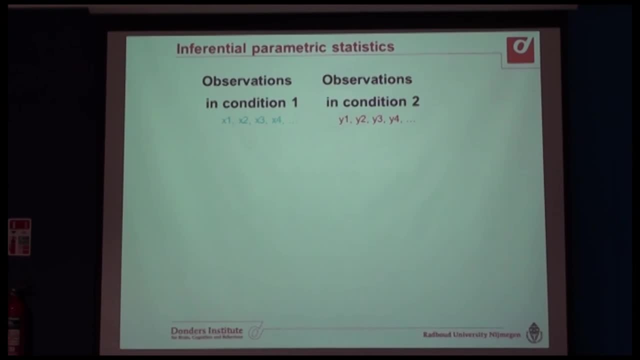 So, rather than comparing to an a priori assumed mean, we often compare the data that is observed into experimental conditions. The idea is the same. We have a distribution of the data in condition X, have a distribution of the data in condition Y. we compute a T-value between them and 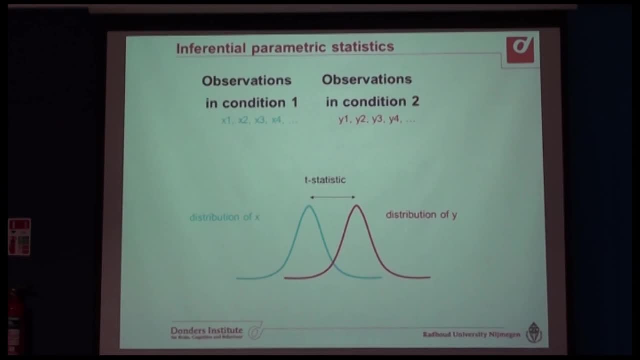 if the T-value is unlikely, given the null hypothesis that the data from both conditions is from the same distribution, then we reject the null hypothesis in favor of the alternative one. Okay, so there's a problem with this and a problem pertaining to MEG data and that. 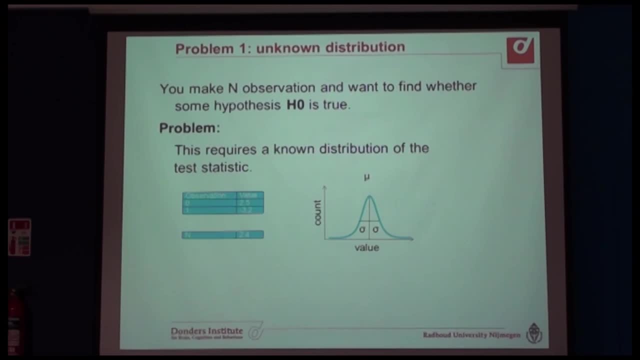 is that it requires a known distribution of the test statistic. So this is nice if our data is normally distributed, but actually quite a lot of the analysis that we're doing on MEG data cause the numbers to be not normally distributed. Power is not normally distributed. 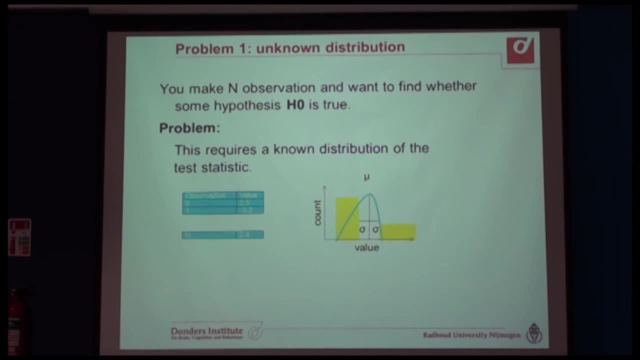 Connectivity values are not normally distributed, So that means that the distributions of the data is not nicely known like this, but it's. for example, it can be skewed towards one side. It has tails which are very different. It might be clipped. Coherence values can never be larger than one, which means that it cannot be normally. 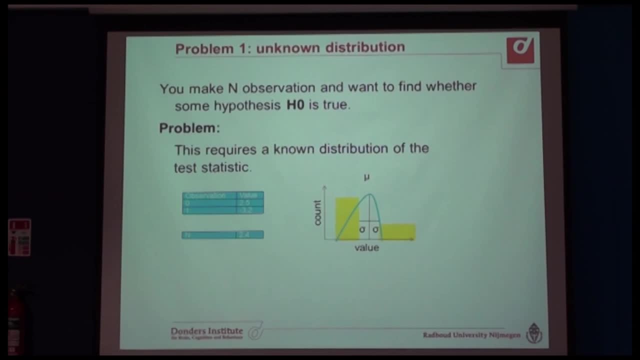 distributed because it's clipped at one. So there's many of these values that we're looking at, that we tend to look at, which cannot be normally distributed. So that means that we're violating the assumptions that are required for a T-test, for an F-test. 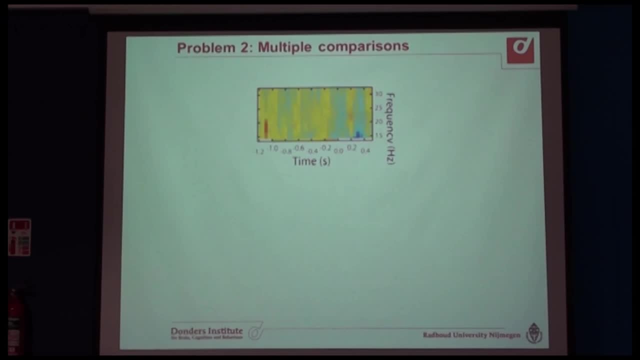 The second problem that we're facing with MEG and with EEG is that of multiple comparisons. So let's look at a single test, So let's look at a single channel where we have a time frequency: decomposition frequency along the horizontal axis, sorry, frequency along the vertical axis, time along the horizontal. 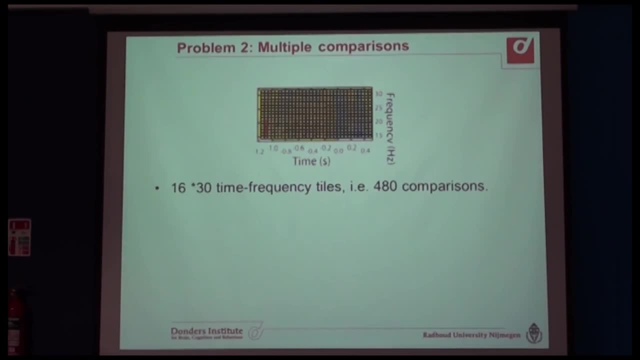 axis. What we actually have is we have many observations in this time frequency plane, So for many time points we've estimated the power at many different frequencies. So let's say that we have 16 frequencies by 30 time points. In total we have 480 points at which we have observed a value over multiple trials in multiple 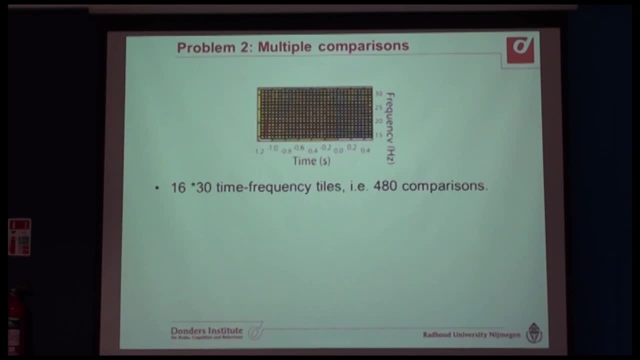 conditions, which means that we're going to do 480 statistical tests. If we test 480 statistical tests with a false alarm rate of 5% for each single test, then we actually have a chance of getting at least one false alarm. that is very close to 100%. 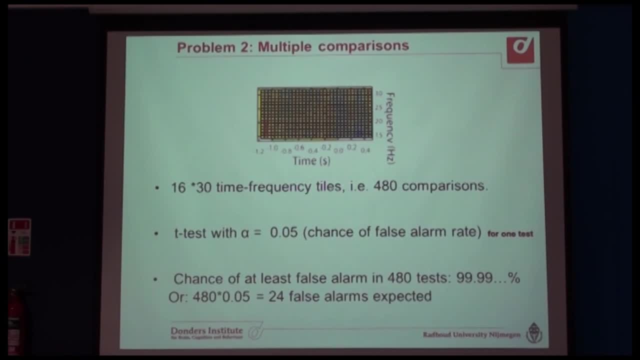 So with so many statistical tests, we would expect 24 false alarms, Of course. did this happen? No, It didn't. So this assumes, like this computation assumes, that all of these tests are independent, which they're not. Like we have spectral leakage, so we know that different frequencies that we're estimating. 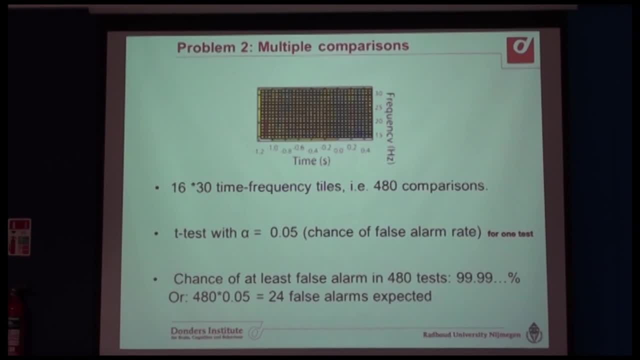 are statistically not independent from each other. We also know that neighboring time points are not independent of each other because we often have these overlapping sliding time windows. But we can also not claim that they're exactly the same, because there are different features visible, so there is some independence in the data. 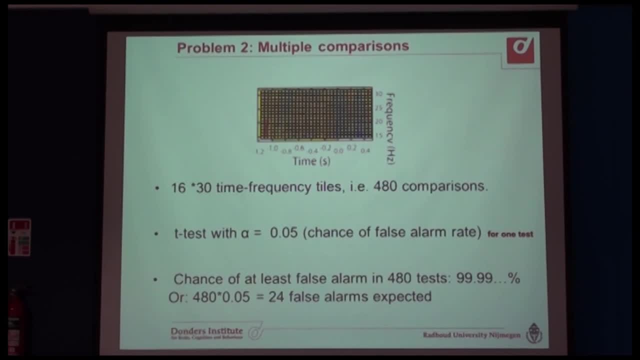 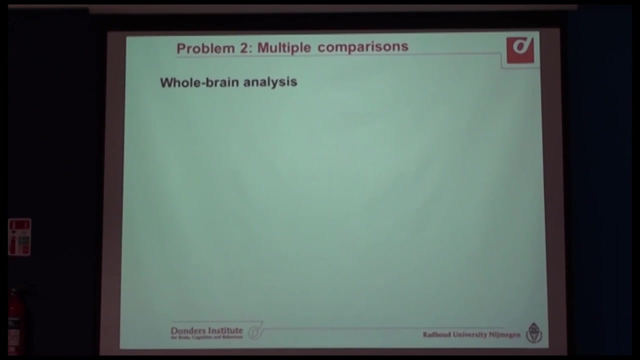 So, although the problem might not be as severe As 24 false alarms, the chances of having a false alarm is actually much larger than the 5% that we're allowing ourselves in reporting these types of findings. The problem gets even greater if we look at the whole brain analysis. 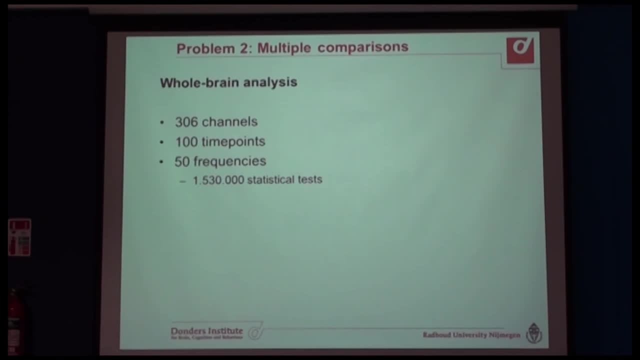 So let's say that we have a Neuromax system with 306 channels, 100 time point, 50 frequencies. This is only like a time frequency analysis of channel level data. that gives 1.5 million statistical tests, Which means that this is the number of false alarms. if we were to assume that all of these 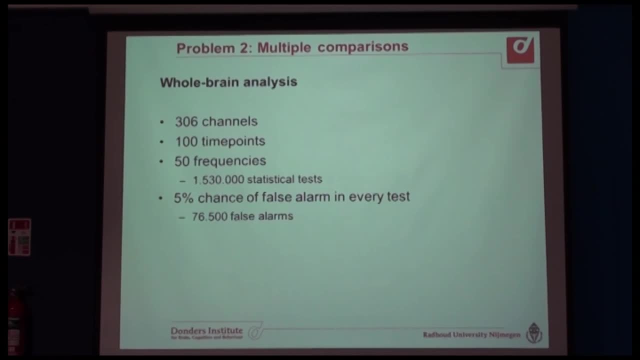 channel time frequency points were independent, So the multiple comparison problem is a serious problem for MEG data. Of course, there are multiple solutions to address the multiple comparison problem, and the one that you're all familiar with is the Bonferroni correction. 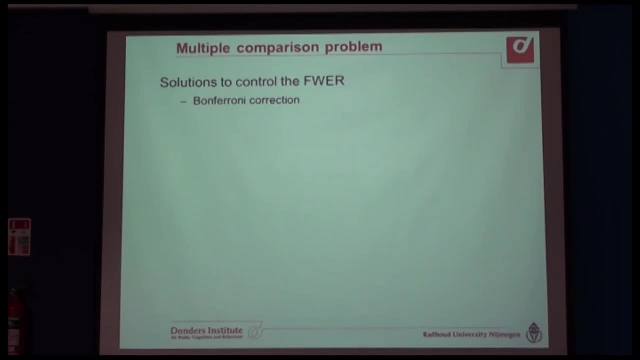 So the idea with Bonferroni correction is If we have two channels, we have a number of false alarms and we have a number of channel time frequency points. If we have two tests and if the chance of having a false alarm in total should be 5%, 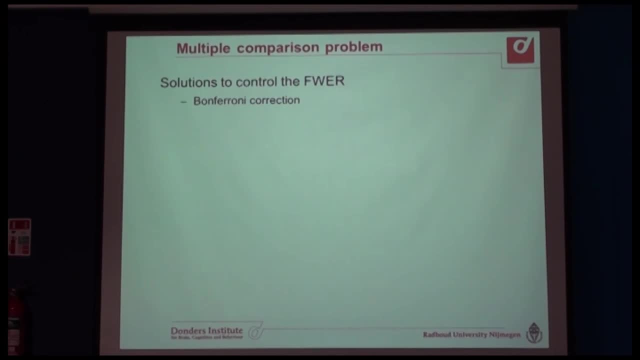 well, let's make the chance of having a false alarm in each of the two tests 2.5%. So we just divide the alpha, the threshold, by the number of tests that we're going to perform. The problem is, if we're going to divide alpha by 1.5 million, then we need to have a really 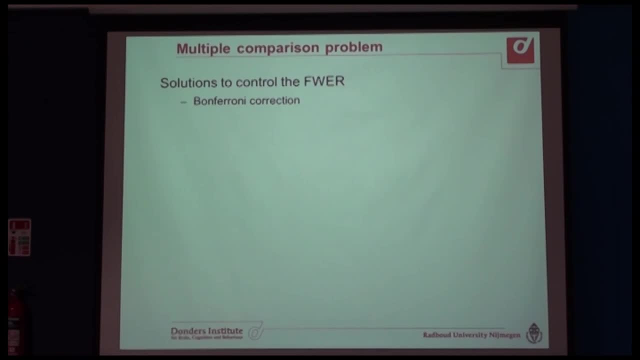 strong effect in order to find it So, Bonferroni, although it's correct, it's not very sensitive, Which means that the chances of us having a false alarm in total should be 5%, And the chances of us having Not being able to report the effect, although there being an effect, is also very large. 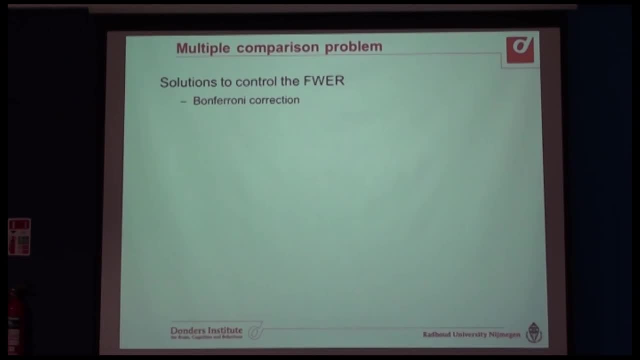 So Bonferroni is Scientifically. it's not a very smart way of going around if you have channel level time frequency analysis and analyze data. The second method that is used a lot is using the false discovery rate, the FDR. 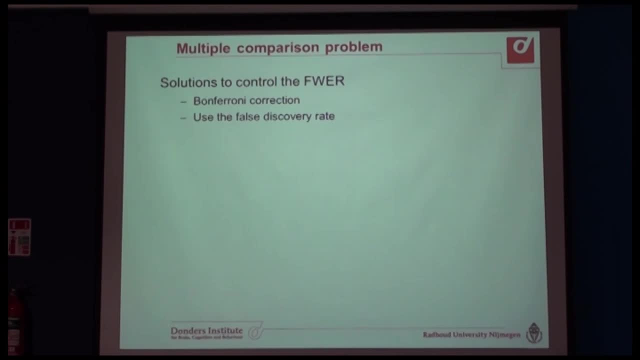 Using the false discovery rate. Actually, we're not controlling the number of false alarms, but we're controlling the expected proportion of false alarms And it's considerably more sensitive than the Bonferroni correction. But the third way, and that's the way that I will explain in more detail in the remainder 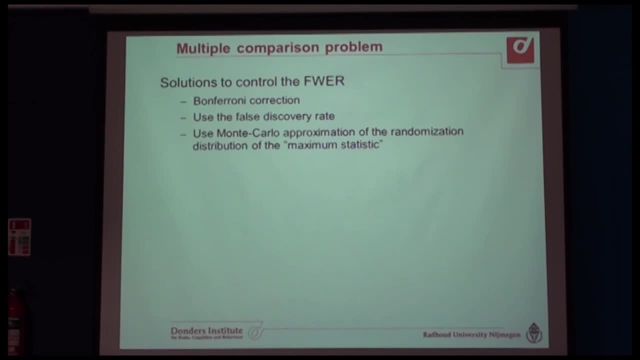 of the talk is to use a Monte Carlo approximation of the randomization distribution of a statistic, And the statistic that we're using is the maximum statistic. All of the words in this sentence will become clearer in the rest of the talk, But I'll just give you a little feel for how that's implemented in fieldtrips. 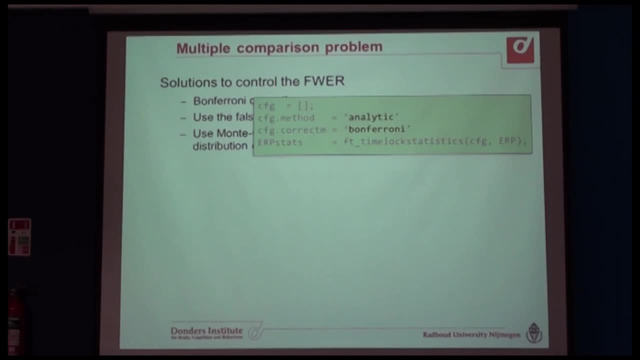 We have functions for statistics, such as FD, time log statistics. What you can specify? you can specify the method, which is the method for computing the probability, And then you can specify the correction for multiple comparisons that you want to use. So, with an analytic computed probability which is, for example, based on t-scores, 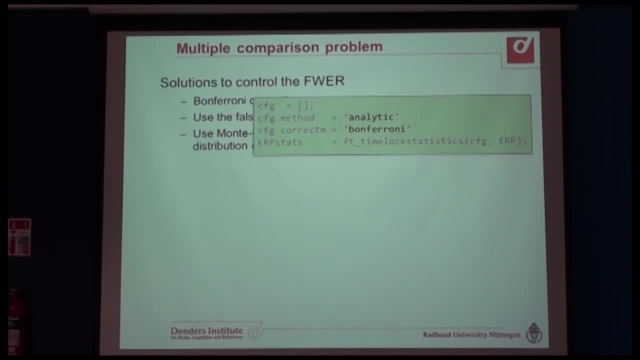 and using a Bonferroni correction. This is how you can configure the function and get a Bonferroni-corrected probability. FDR is basically the same. The only thing that you change is the CFGcorrectM field in the configuration. 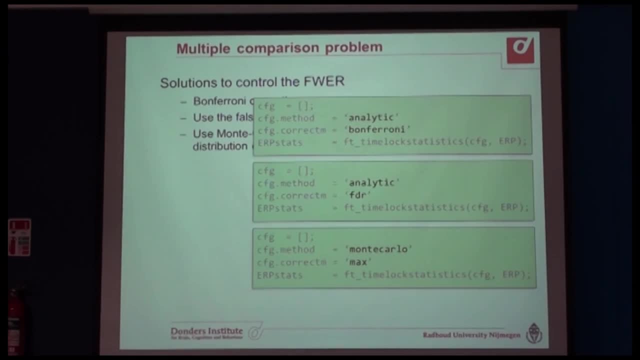 And if you want to do a Monte Carlo statistic. so, rather than specifying analytic, you specify that you want to use the Monte Carlo method for estimating the probability And you can specify that you want to use the maximum statistic for controlling for false alarms. 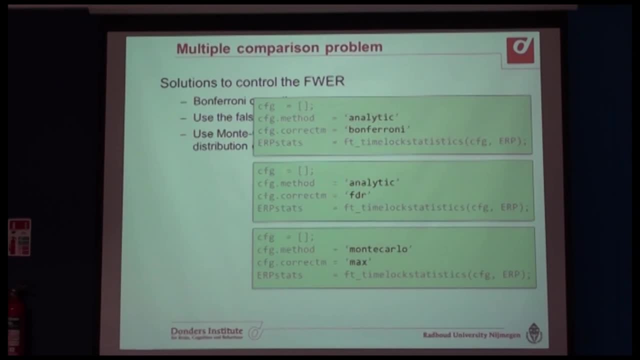 What you see here is that I'm showing FT-Timelock statistics. Basically, we have three functions that serve as entry points. So we have FT-Timelock statistics, FT-Frag statistics and FT-Source statistics And the functions. they only differ in the way that they do the data bookkeeping. 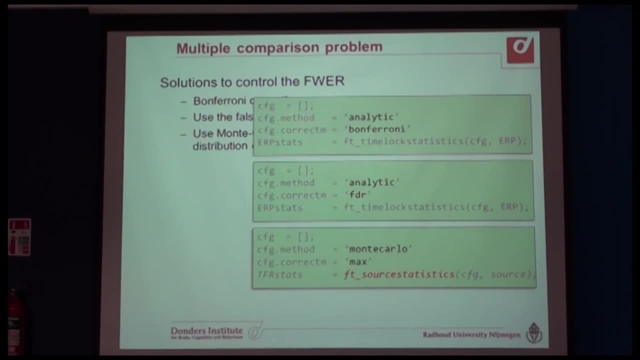 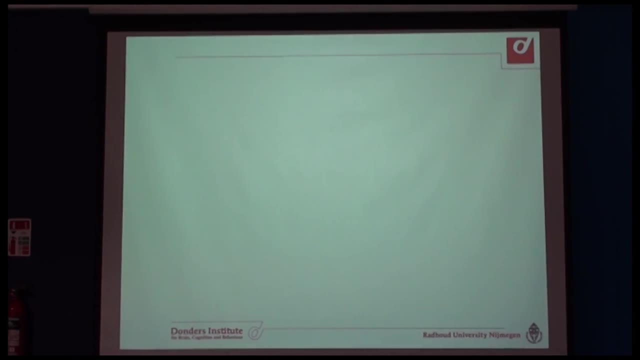 The underlying machinery is the same for the three functions, But it's basically just different, Different data structures that they take Clear. so far, Okay. so the general principle of a randomization test is that we consider the data. We have an independent variable and we have a dependent variable. 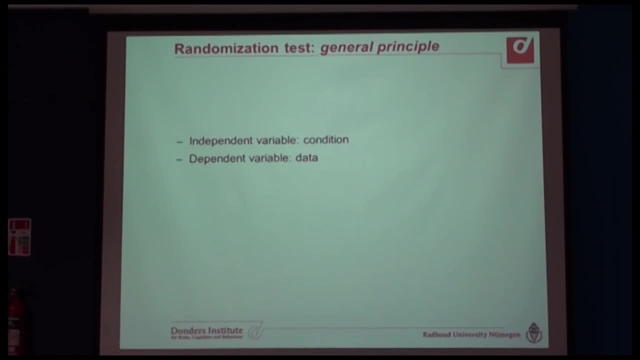 So the independent variable is the one that you've experimentally manipulated as the condition in which you observe the data, And what we assume is that the data depends on the condition in which the data was observed, So that means that we can phrase a null hypothesis. 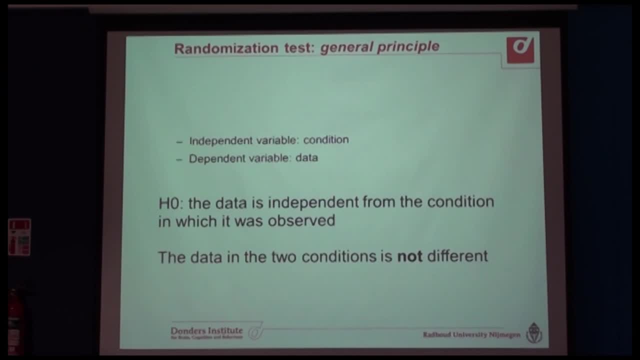 And the null hypothesis is that the data is independent from the condition in which it was observed. So the null hypothesis is basically: the brain is doing whatever the brain is doing, but it doesn't really care about the stimuli that you are presenting. And you can rephrase this: 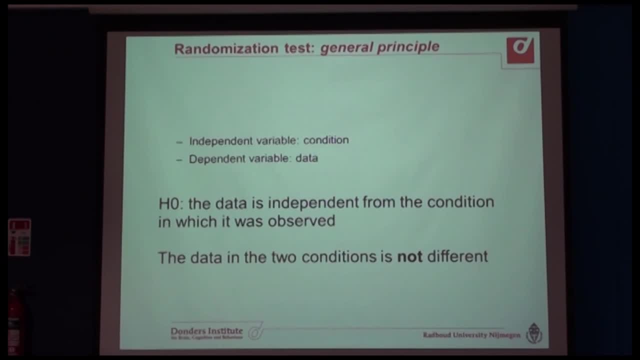 You could say: the data in the two conditions is not different And if we believe this null hypothesis, well then we can. basically, we can use this schema So we can take the data in one condition, we can take the data in another condition. 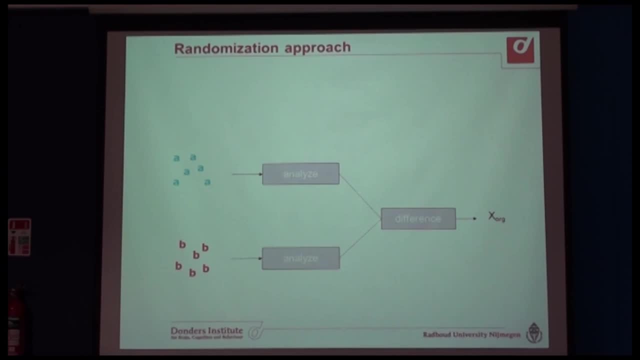 we can analyze it and we can compute some sort of a difference. And the analysis that we, for example, perform is the computation of mean value and the computation of the variance or the standard deviation, And the difference is, for example, computed by taking the difference between the means. 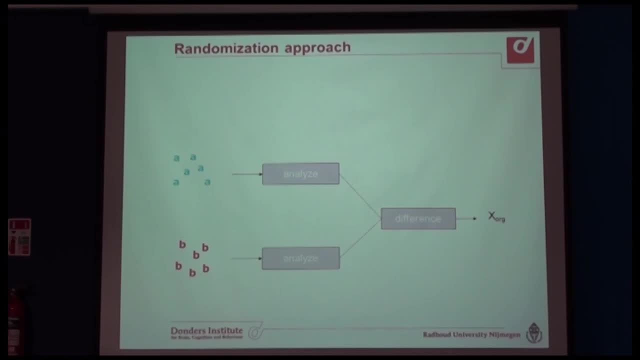 divided by the estimate of the standard deviation. So that means that we get a number out and this number is the statistic. But under the null hypothesis we can- actually we can- shuffle the data over the two observations. So rather than keeping this data here and here, 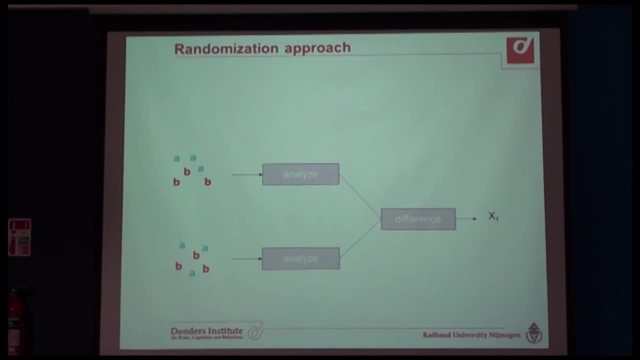 I'm just going to shuffle between the two pools And I'm again going to compute the mean and the standard deviation and I'm again going to compute the statistic. And that is something that I can do many times And for every time that I compute this statistic. 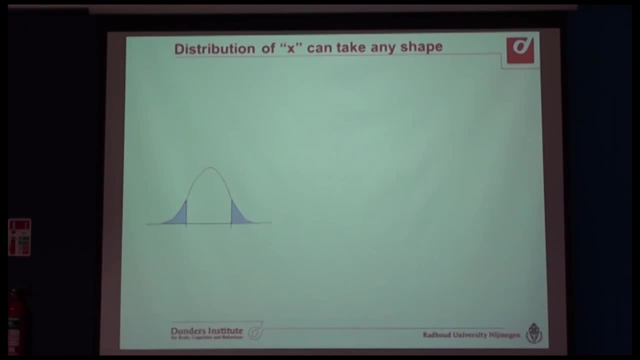 I'm going to store it, I'm going to make a histogram out of it and afterwards I can, I can, I can look at this histogram. So that's the Monte Carlo approach of sampling this distribution. So it's the Monte Carlo sampled distribution. 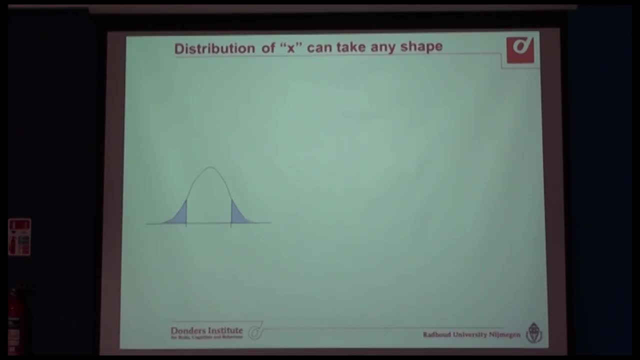 of the randomization distribution of the statistic of interest. The interesting feature is that I don't have to make an a priori assumption on how this distribution is, because I'm estimating it from the data, And that also means that the distribution can take an arbitrary shape. 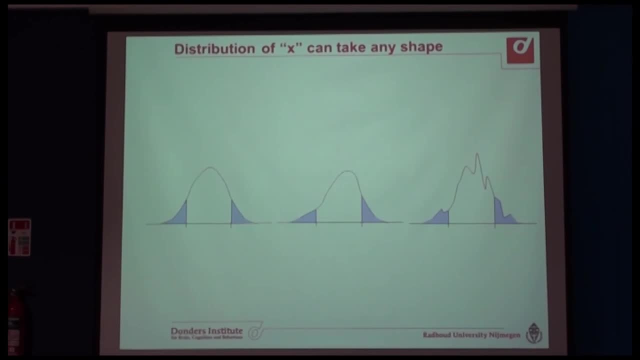 So it can be skewed and it can actually, it can be random, But what we expect is that, under the null hypothesis, the statistic that we observed, given the data in our original assignment of the data, should be somewhere in the middle of this distribution. 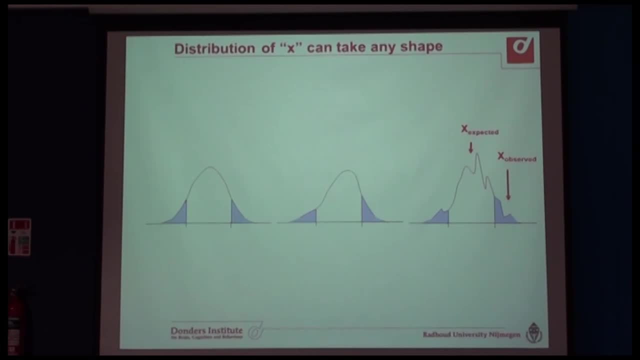 And if the statistic that we've observed for the original assignment of the data over the two conditions is in one of the tails of the distribution, then actually we consider the null hypothesis to be very unlikely And we would reject the null hypothesis. So this is this is this is independent. 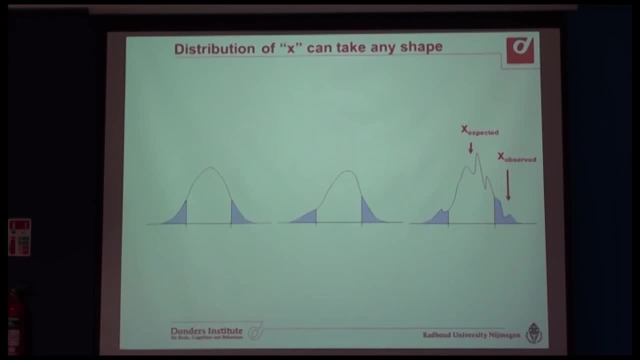 or? this does not depend on the distribution of the of the statistic. We're estimating the statistical, the distribution of the statistic, and we look whether the observed statistical value falls in one of the two tails of this distribution. Is this clear? The nice thing is that, although we can like 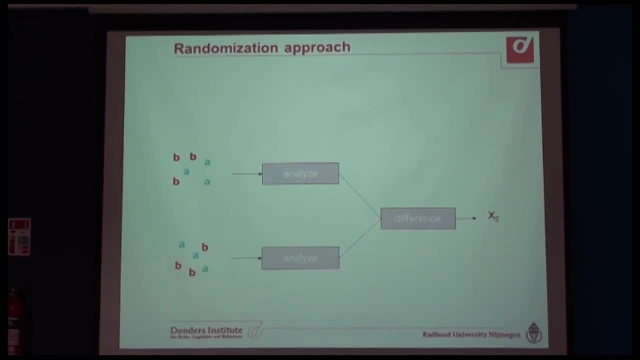 compute mean and we can compute variance, but the procedure does not depend on what we're doing in the analysis. So basically we can plug in any black box and as long as we have our data and as long as we're computing some sort of a difference. 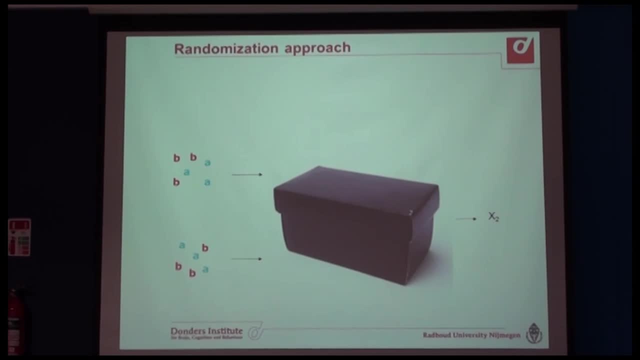 the procedure holds, because the procedure does not make any assumptions about the distribution. the procedure only makes an assumption about the similarity of the data over the two conditions, Because that's the null hypothesis. So you you can, for example, compute the difference as the. 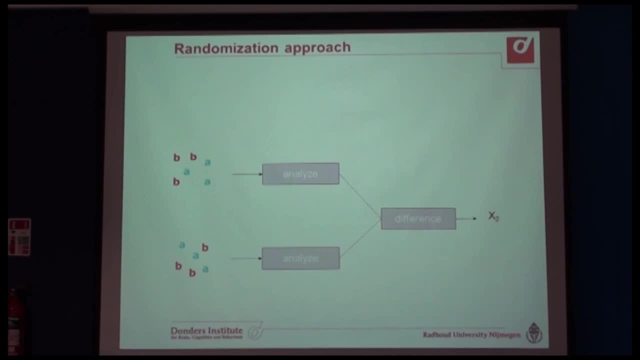 the difference between the mean divided by the standard deviation. but you could also just compute the difference in the means. you can compute a ratio. you can anything like. usually we would do permutation, but it but it depends on how the experiment was designed. so usually we will permute the data that was observed in each of the conditions over the two possible. 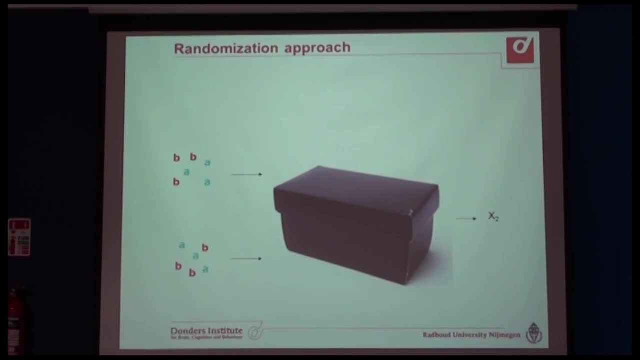 conditions. so that means that, like yesterday we've already shortly touched upon like: how do you deal with um experimental designs where you have different trial numbers in each of the two conditions? so let's say let's, let's give, give, let's assume that we have, we've observed the 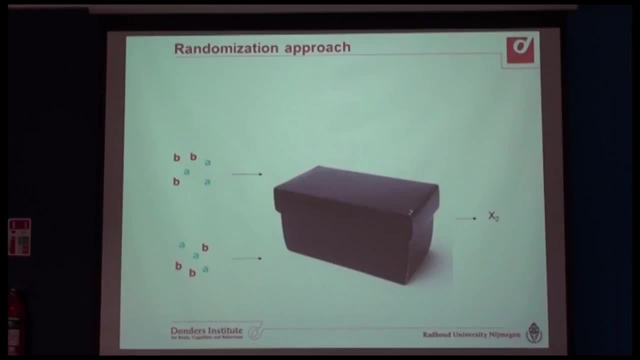 data in 100 trials. we have 70 trials in this condition and 30 trials in this condition. as long as i keep the number of trials in each of the two conditions the same- but i just shuffle the data between the two conditions- i'm always going to keep. 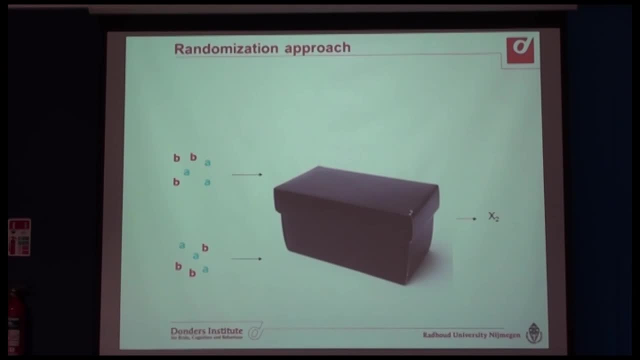 70 trials here and 30 trials here. that means if the numbers that i'm computing, the numbers that i'm analyzing in this black box, say coherence, if those numbers are biased, coherence is biased by the number of trials. like the fewer trials the higher the coherence will be. then also that bias. 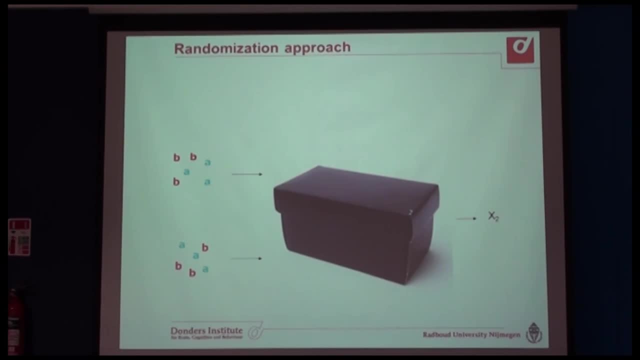 is going to be reflected in, let's say, the difference in the coherence. like the condition with 30 trials is always under another hypothesis, it's always going to have a larger coherence. but that means that the randomization distribution is actually going to reflect this bias as well. 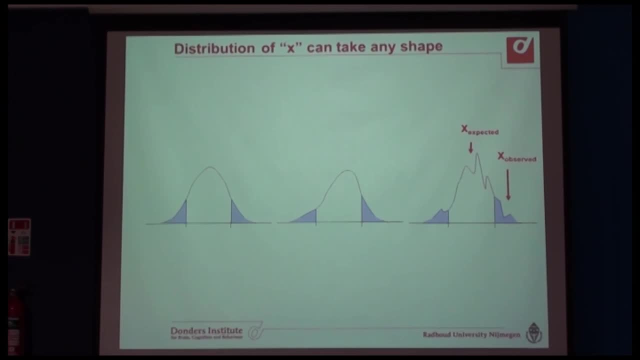 so that means that if we permute, we don't care about the bias, as long as we keep the same number of observations in each experimental condition. so that's why we normally permute. uh, it's also possible to randomly reassign, but that's um, but that's the we, we fields of can do that, but 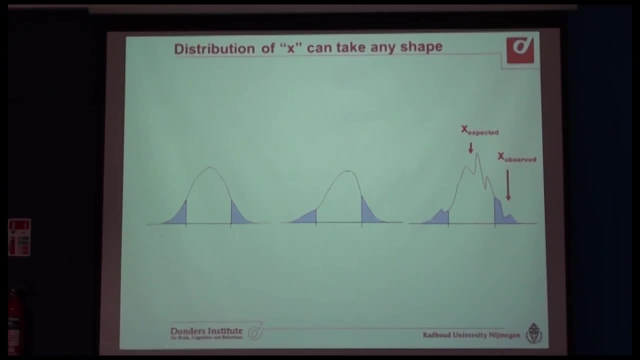 we general. we in general we permute. permutation is just a subset of randomization distribution, so we're only taking a subset of all the possible randomizations. usually we do approximate permutation because the number of permutation is too large to do an exhaustive search and that's also why we call it the monte carlo approximation of the randomization. 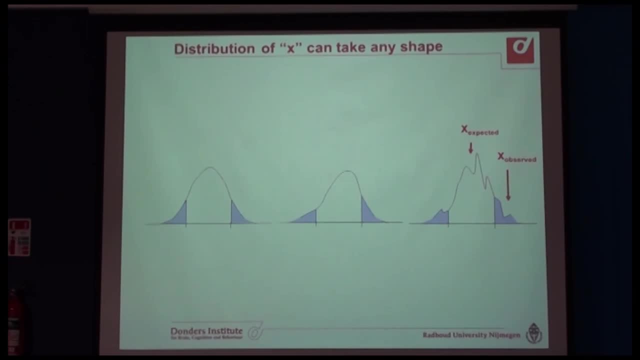 distribution, because we're only taking a subset of all the possible randomizations. there are cases where the number of permutations, the number of possible permutations, is not that large and in that, in those cases, we will actually do where we, we will compute all possible. so both are possible. it depends on, like this, the size of your sample. 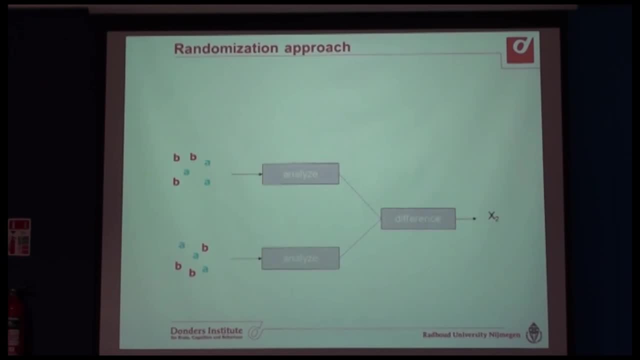 yeah, okay, so the yep: well it's, it's, it's. the more permutations you do, the the better the approximation is going to be, uh, but also the longer the time it's going to take, uh, so, so, so we, we, when we, when we started doing this uh five years ago, we, 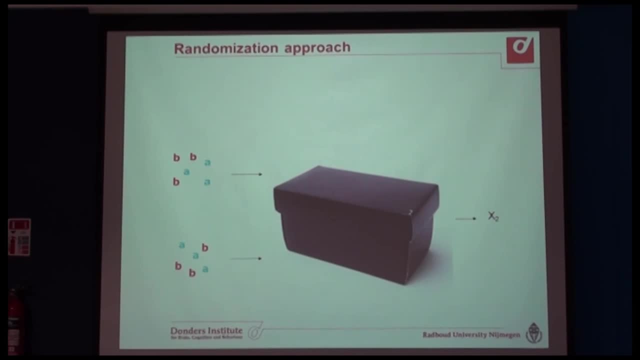 we used to do 500 permutations because that was just manageable. yeah, but like with these large data sets, it was just manageable, uh, since then we've of course gotten bigger computers, so now we would by start, by default, do like a thousand permutations. um, recently there was a paper i've 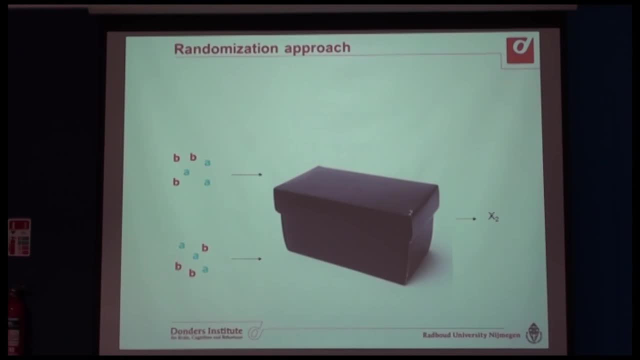 forgotten which journal it was it. it was from uh, guillaume, russia, and um and as and so so from from glasgow and from edinburgh. they looked at the number of permutations. they also compared to different methods for uh permutations versus randomizations, versus bootstrapping, um and the, the. their conclusion was that the defaults that were 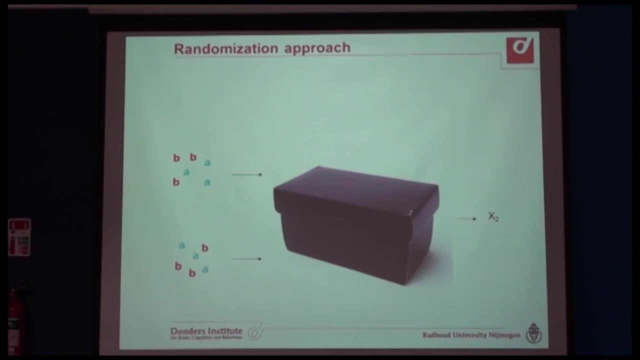 that we have in field trip are actually quite okay like they're. they are almost as sensitive as the best method, uh, and, and they're quite manageable? um, i don't think so. um, yes, if you want to have the paper, just send me an email. i'll look it up for you. 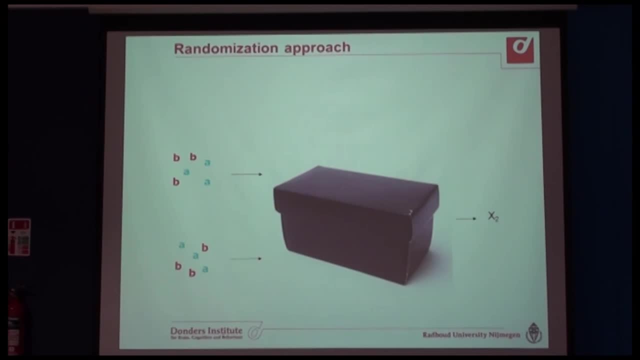 okay. so, of course, like, the more permutations you do, the more accurate it becomes, and it's your responsibility to be confident about your claims. so if you don't feel comfortable about doing a thousand, well then do ten thousand or a hundred thousand. uh, it just depends what the 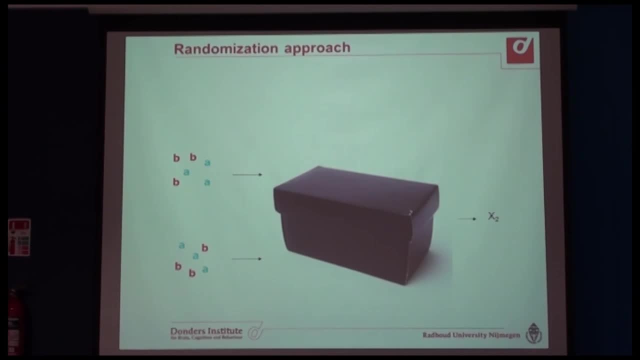 whether we, whether you can fit all of this in the in memory because it's it is a bit memoryy intense. okay, so the idea is that we randomize the independent variable. so we say we basically break the linkage between the condition and the data and then we shuffle, but the hypothesis that we're phrasing is a hypothesis about the data. 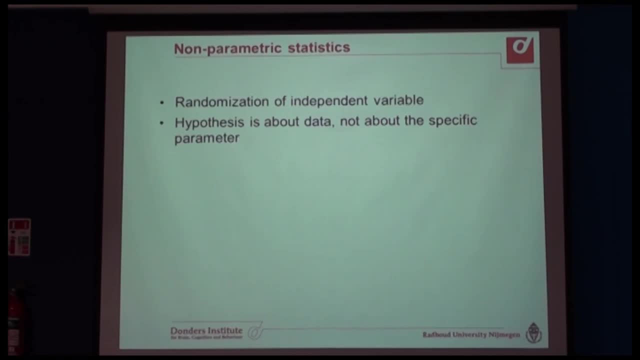 it's not about a specific parameter that we're computing out of the data. so basically, this black box can can compute any parameter. we can compute the difference with the difference in that parameter between any two conditions, um, and then the randomization distribution is approximated using a monte carlo approach, where 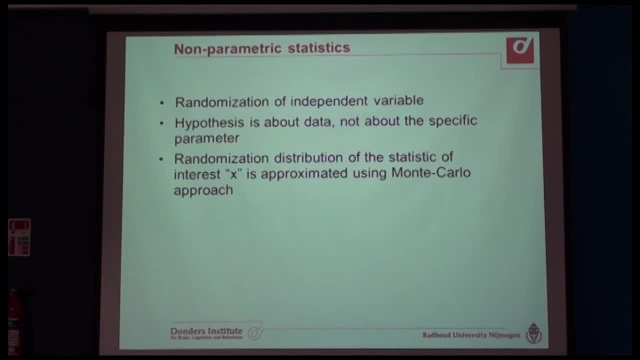 we take a subset of all possible permutations, or we do an exhaustive, like we compute all possible permutations and then, uh yeah, so the null hypothesis is is tested by comparing the observed statistic versus randomization distribution. so how does this help us in doing statistics? well, one thing that it does is that it allows us to 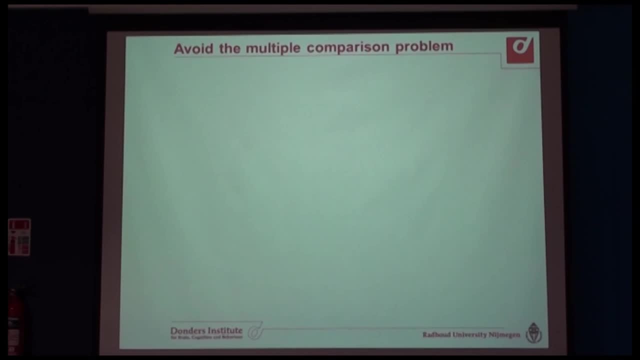 make inference independent on the distribution of the statistics. so we it works for, for power, it works for clearance or for other weird measures that we might be deriving from our energy data, but actually has much, much more relevant aspect to it, which is that it allows us to avoid the multiple 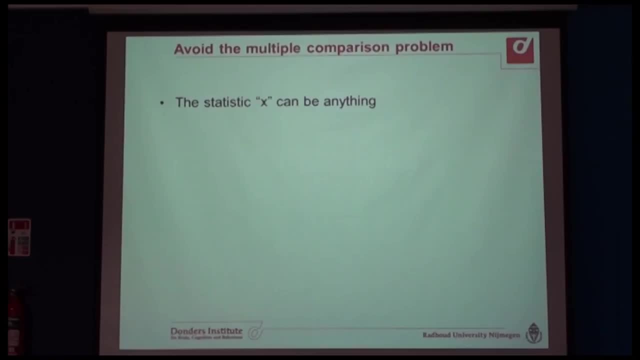 comparison problem, since the statistic that we're computing can be anything. what we can do is we can, rather than test everything, we can test the most extreme observation. so, rather than basically looking everywhere in the brain, we're just going to look at the location where we have the most extreme. 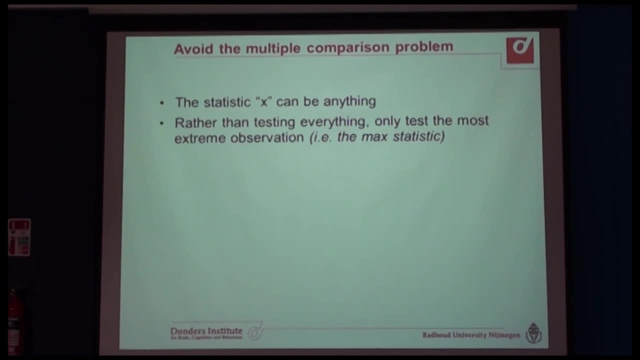 difference between the two conditions or where we have the most extreme difference between the two pseudo conditions after shuffling the data. so what we do in general is that we compute a randomization distribution for the most extreme statistic. if the most extreme statistic is unlikely, then the 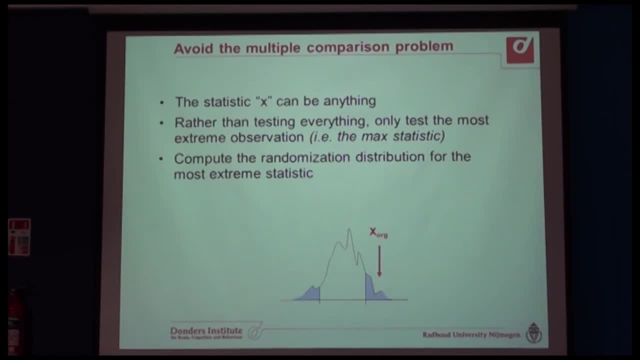 null hypothesis is rejected. there is one catch here, and that's often we have a question in which we don't know whether the effect is going to be that the data in one condition is going to be larger or that the data in the other condition is going to be smaller. so what? 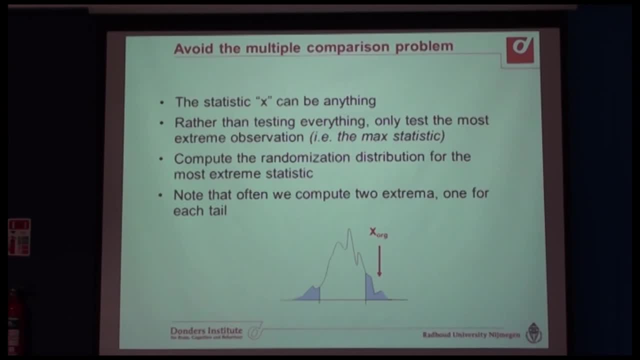 we often do is we have two tails that we have to consider. so if I'm saying we're computing the maximum statistic or if I'm saying I'm computing the most extreme statistic, what we usually do is we compute the most extreme positive statistic and the most extreme positive statistic and the most extreme positive 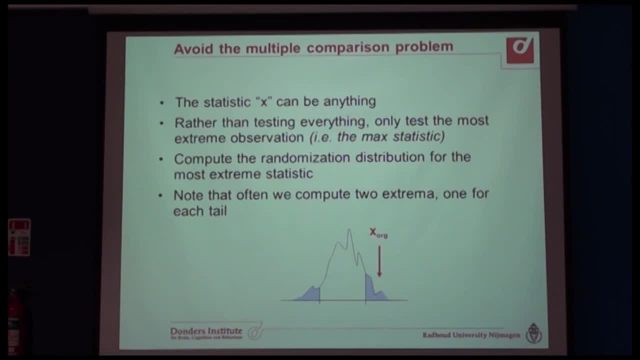 statistic and the most extreme negative statistic, which means that we're actually we're doing two randomization tests, one for the most extreme positive, one for the most extreme negative, and we're correcting for those permutation tests using one-for-only correction allowing for two and a half percent on. 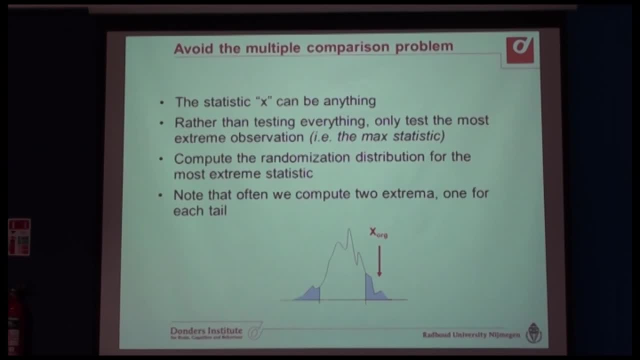 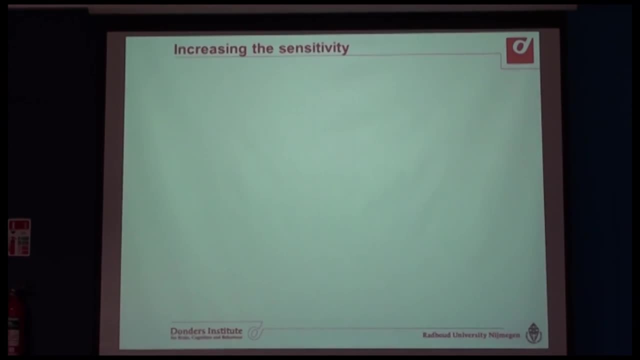 one side of the distribution and two and a half percent for the other side of the distribution. yeah, okay, so I've shown you that the randomization, that nonparametric testing using a randomization approach, can be used to test data for which we do not know the distribution, and that we 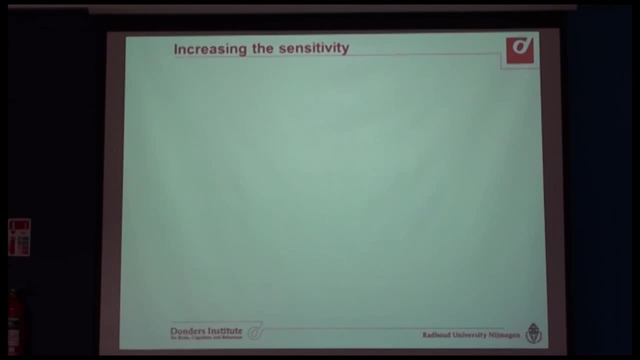 can use it to circumvent the multiple comparison, multiple comparison problem. what it also allows us to do is to increase the sensitivity, and that's, of course, very important. so the conventional way of doing statistics is to do a massive univariate parametric test, and our approach is to consider the 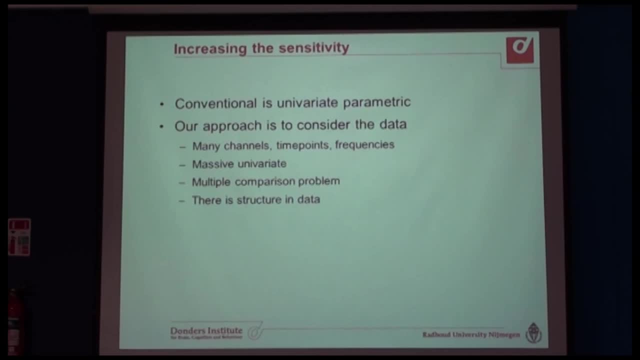 data, Like we know that in this channel time frequency data that neighboring channels show the same thing. Neighboring frequency points, they also show the same thing. So what we're doing is we're using the structure that is present in the data to increase the sensitivity. 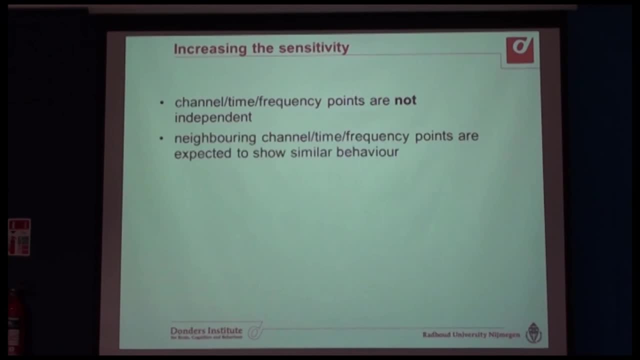 And increasing the sensitivity is done by using our knowledge about the data, about the data being like neighboring channel time frequency points showing the same thing. So what we do is we cluster them, And you can think of this as that we're accumulating evidence. 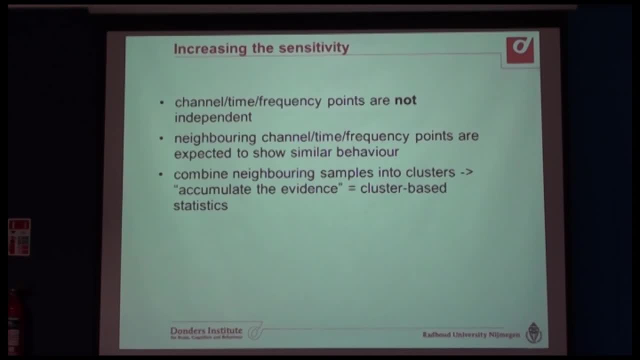 If one channel is showing an effect, if a neighboring channel is also showing the same effect, well then we consider that to give additional evidence that there's something going on on those channels or on those brain locations after source analysis. And the same goes with time and with the frequency domain. 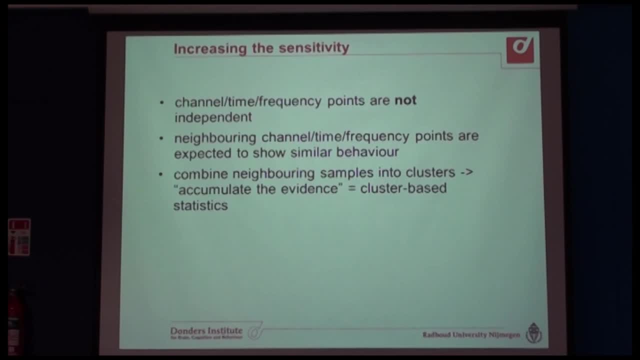 We know that there are estimates in the frequency domain, that they're spectrally smooth, That there is spectral leakage. So rather than say well, each estimate is independent from each other, we just say: well, each estimate is not independent of each other. 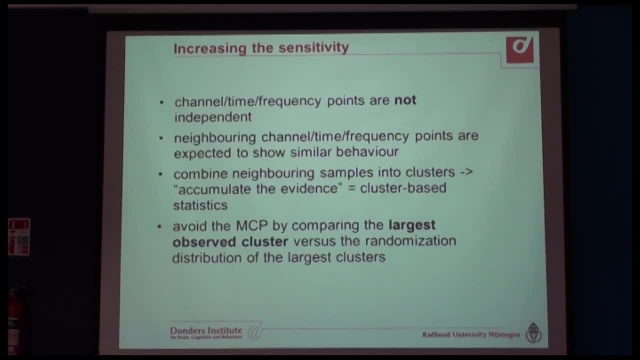 We expect structure And again we're avoiding the multiple comparison problem by comparing the largest observed cluster versus the randomization distribution of the largest clusters. So we're still using the maximum statistic or the most extreme statistic, But that's not the most extreme observation. 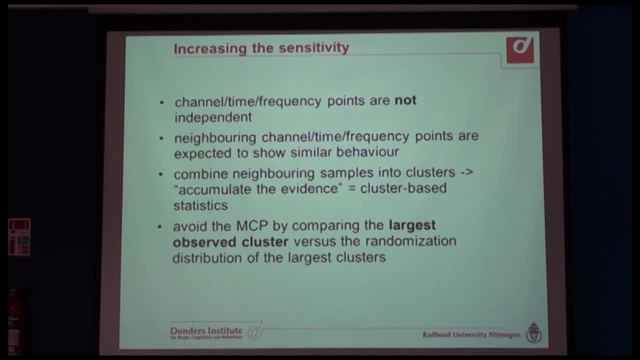 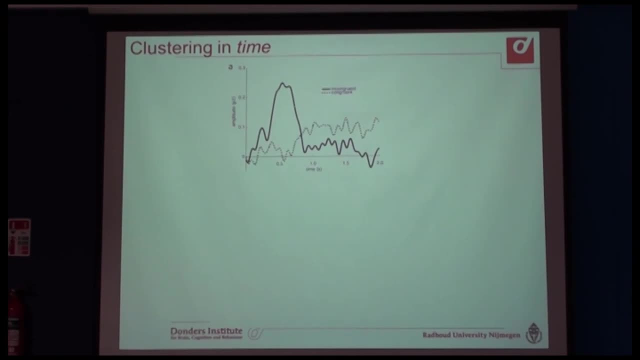 but it's the most extreme cluster, So let me explain this in a bit more detail with the data that we started off with on Wednesday afternoon. So it's the language task, And what we've already shown is that about 400 milliseconds after the onset of an unexpected word in a sentence, 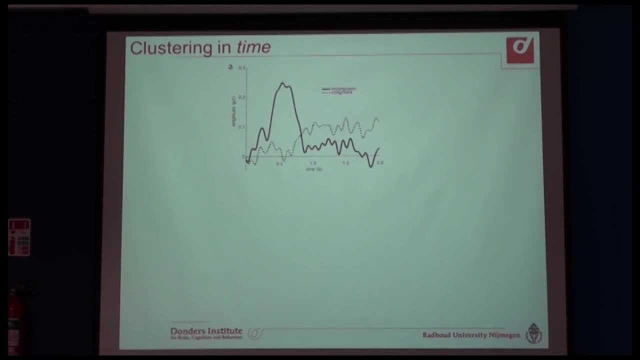 there is an N400 effect. So what you see here is the congruent and the incongruent condition, And what we can do is we can for each time point. so this is a hand-picked channel for each time point. 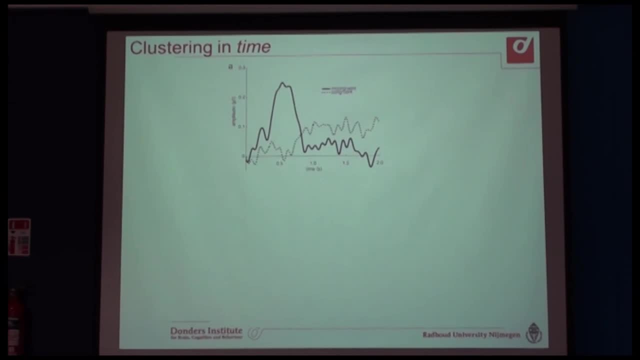 we can compute, OK, The mean value. in both conditions. we'll compute variance and we can compute a t-score. So what I show here is actually the t-statistic for each of the time points, And what we can do is we can threshold the t-statistic. 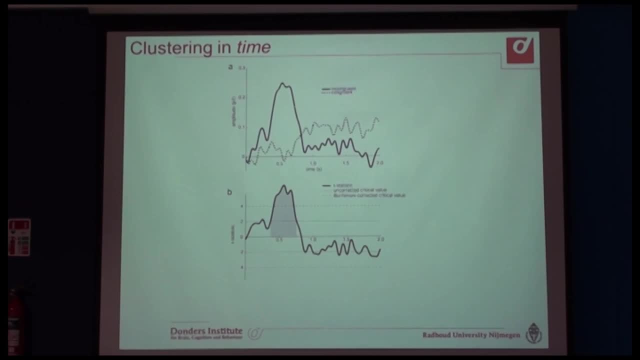 So if we threshold it without considering multiple comparisons, we would set the threshold approximately at plus 2 and at minus 2. And that would result in these time windows where the data indicates It indicates there to be a significant effect. So there's actually quite a lot of time windows. short snippets: 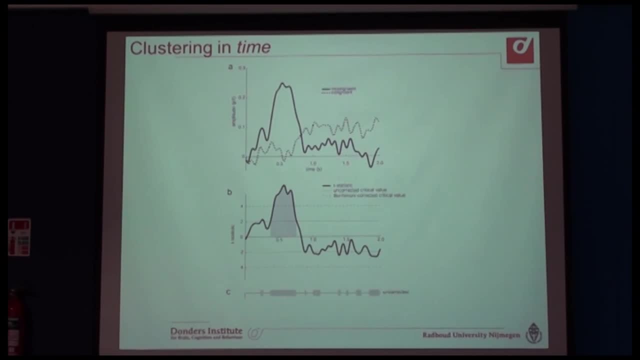 in time where the data exceeds this plus 2 or minus 2 threshold. If we do a multiple comparison correction, we can correct for the number of time points, which I think is about 300 or so, And we can correct the alpha level. 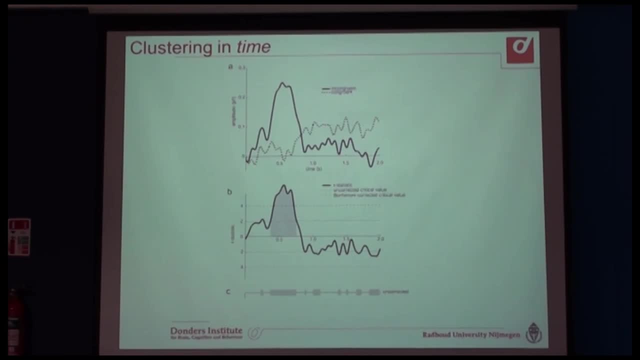 Given that alpha level, we can compute the critical t-value, And that critical t-value happens to be 4.. So if we do a point-to-point correction, if we do a Bonferroni correction, then only this part of the data exceeds the a priori threshold. 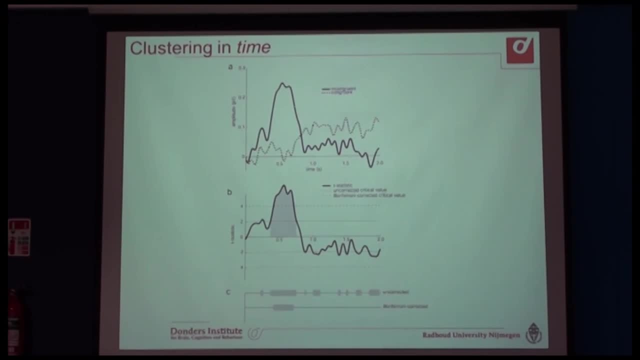 So that's fine. So that means that with a Bonferroni correction we can show that there's a significant effect. But what we do is we basically take clusters. So what we do is we take the initial, a priori chosen threshold of 2.. 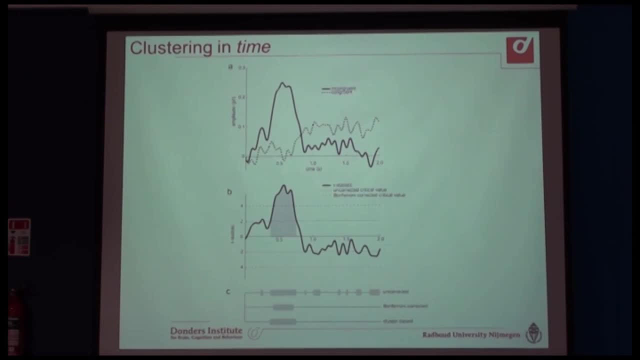 And for each of the time windows we compute the area under the curve. So for each of these small snippets where it exceeds the threshold, we compute the number of time points and the t-value in each time point we add that up. 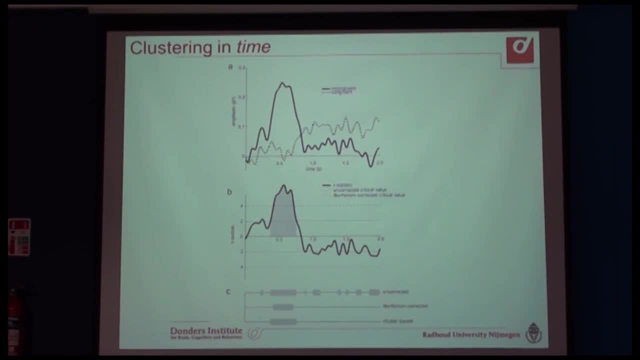 We integrate it for each of the clusters And then we take the cluster that has the largest sum of t-values, We store that in a distribution And then we randomly shuffle the data And we can compute the largest cluster, et cetera, et cetera. 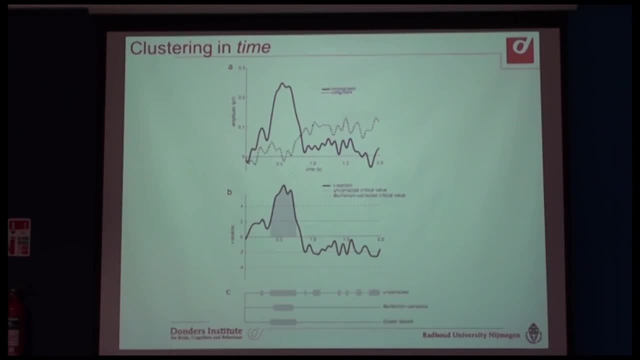 And then the cluster. so the largest cluster which is indicated here in gray is very unlikely, given the null hypothesis of the data being exchangeable. So actually the gain that we have in this data is very small because, if I do a Bonferroni correction, 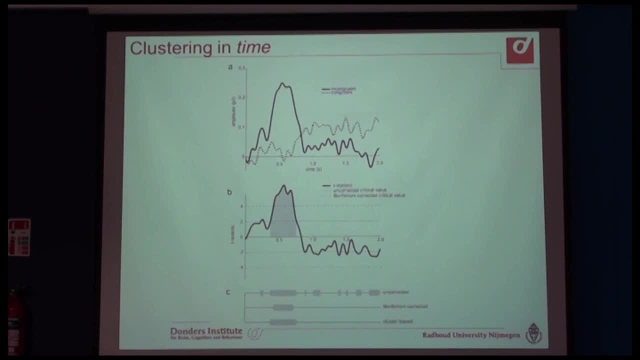 it's significant And if I do a cluster-based statistical test, it's also significant. But here I'm cheating because I've already hand-picked a channel And of course I've picked the channel with the largest effect, which is not fair on a null hypothesis. 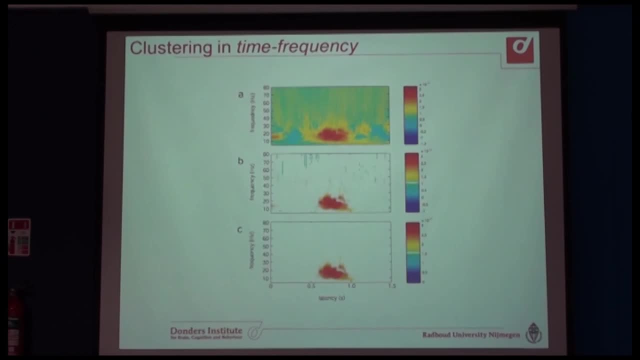 Like on a null hypothesis state: well, there's no effect. So let's now look at the time frequency data. So, basically, this is one of the results from the hands-on session that you did yesterday morning, So this is again. it's a hand-picked channel. 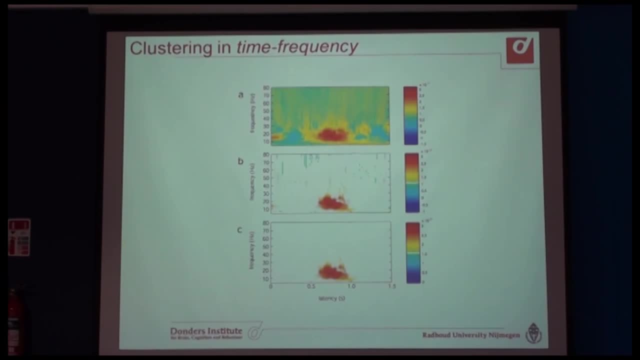 We have the time frequency domain And what we can do is that now plotting gets a bit more difficult. But what we can do is we can again compute a t-statistic And we can threshold the t-statistic to get a binary image. 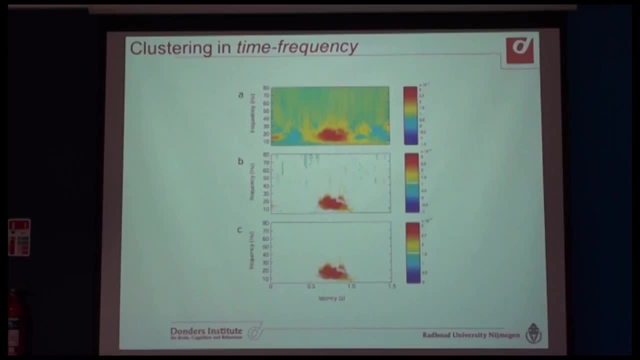 And what I'm showing here is the t-statistic. sorry, is the effect thresholded using the t-statistic without correcting for multiple comparisons. So then, what you see is that there's multiple small points, like patches, and one large patch at which the t-statistic 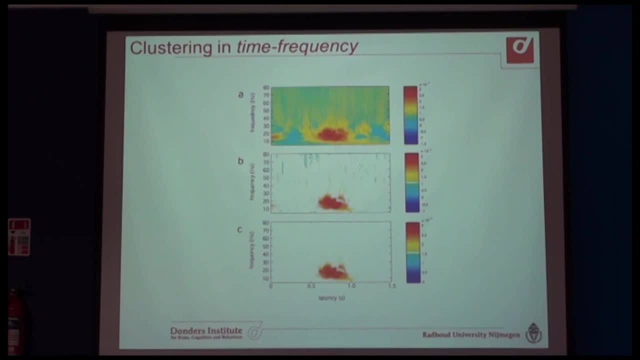 exceeds the a priori chosen threshold. The t-statistic is basically what we've put in the box. Like you can use an a-bit trace statistic For the T. the reason why we're quite often using the T-statistic is because we know 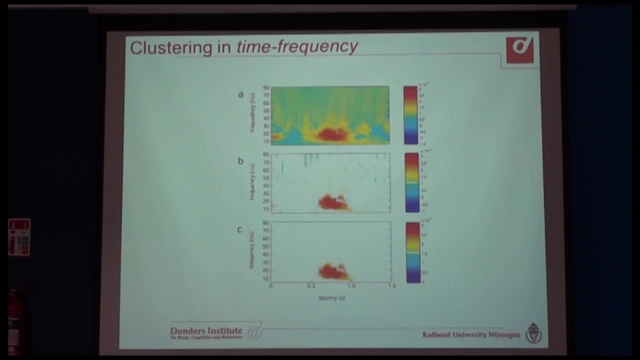 reasonably well how the T-statistic behaves. So we know that we can have an a priori threshold of two and minus two. You can also take another statistic, but the T-statistic is just one that we happen to know quite well. So the procedure works independent of the statistic. 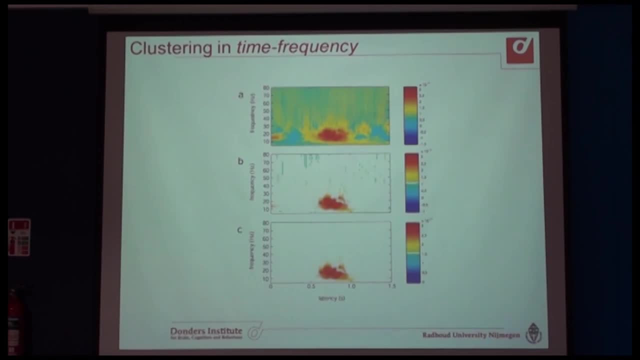 but the massive univariate statistic we usually take is the T-statistic. For each randomization. we compute the T-statistic at each channel, time, frequency point And that T-statistic is thresholded, and then, given the thresholded data, 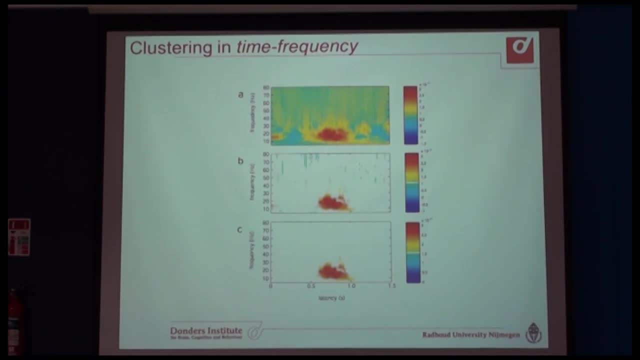 this will hopefully become clear in a few slides from now, but then, given the thresholded data, we identify the clusters and then, for each cluster, we compute the weight in that cluster And it will become clear in the few slides from now. Okay, so this is the data thresholded at a T-value of two. 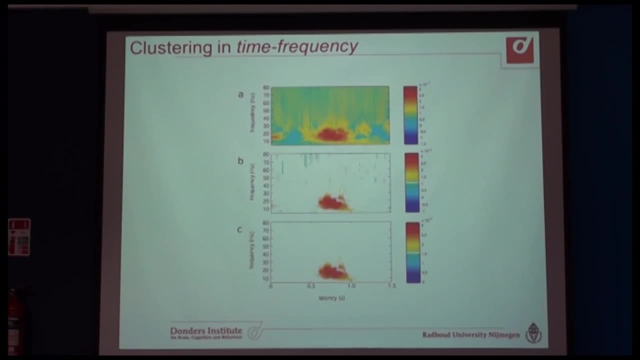 If we apply a bond for all the correction here, then none of that time frequency point actually has a T-value that is sufficiently large to exceed the threshold. If we do the cluster-based test, then this is the cluster that is unlikely, given a null hypothesis. 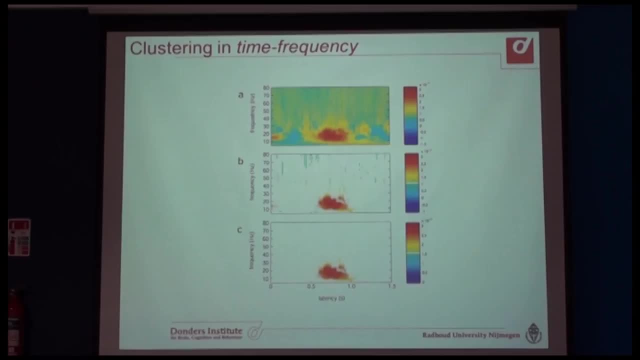 So already with single-channel tests, which are extremely rare, these are the clusters that are unlikely to get a null hypothesis. So already with single-channel tests- time-frequency data- the cluster-based test is clearly outperforming a Bolt-Frohny correction. 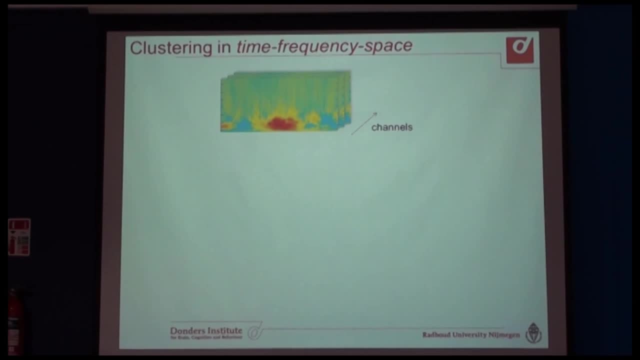 And the situation gets even more obvious that this is a very sensitive test. if we move to channel time-frequency, so if we also add a channel dimension, Visualizing the data gets a bit challenging because these clusters, they basically have a spatial, a temporal and a frequency aspect to them. 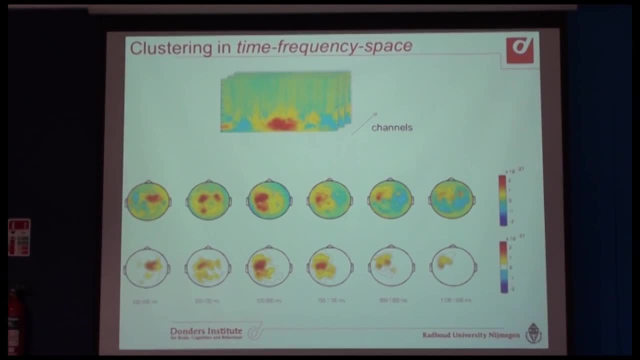 So what we can do is we can again here for specific time windows. I'm now zooming in on the beta effect. so what I've done is I've, for specific time windows, I've plotted the spatial topography in the beta bands and what you see is that the beta topography 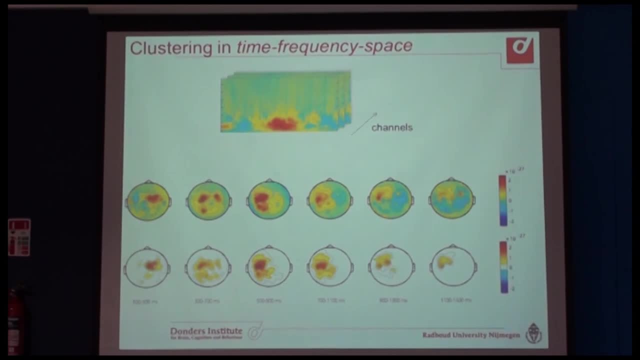 is changing over time. We can compute T-values, we can threshold this, and there is this cluster that is exceeding the threshold. So one thing that you might notice: Notice that this is not really a physiologically interpretable cluster, because it starts. 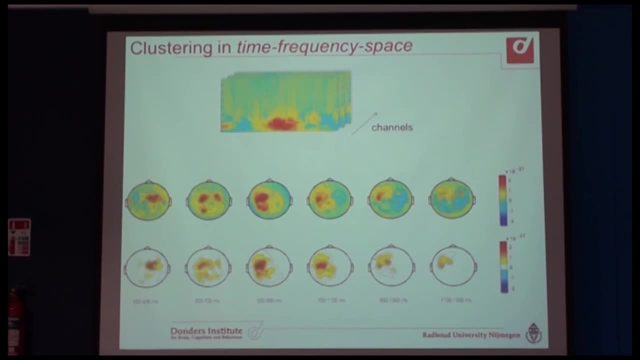 like at early latencies on the right side and then it moves towards the left side. But we're not making assumptions that the clusters are physiologically interpretable. The cluster is just what we put inside the black box and the method is valid regardless. 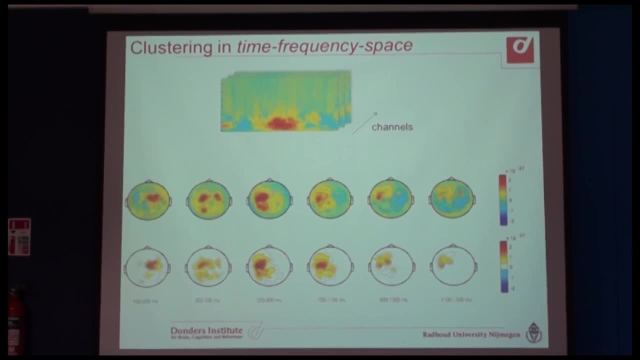 of what's in the black box, So we can put physiologically meaningful stuff in the black box And of course, these clusters can have some interpretation. but I think it's important that you realize that you should not be interpreting the clusters. 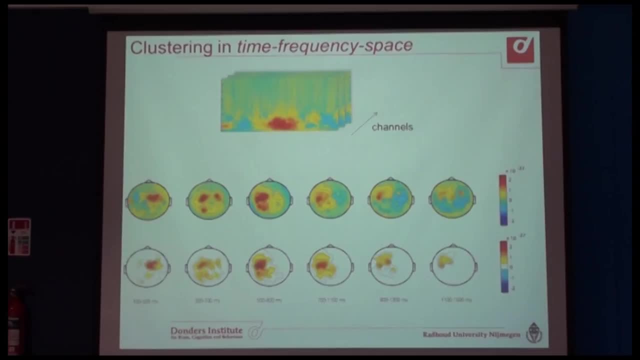 You should be interpreting the data. The statistic is. the statistical test is a test about the data. It's not a statistical test about the clusters We're just using, we're exploiting the clusters to increase sensitivity. So give me a. to give a toy example: 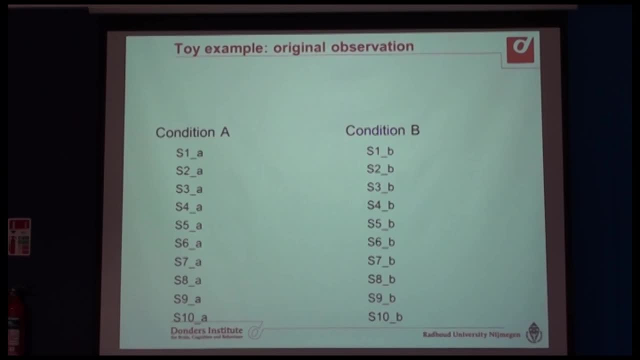 So what we have? let's say we have observed 10 different subjects in a condition A and a condition B. Uh, For each of them we have an event-related potential or a time-frequency distribution, And what we do is we randomly shuffle. so, under the null hypothesis, the conditions. 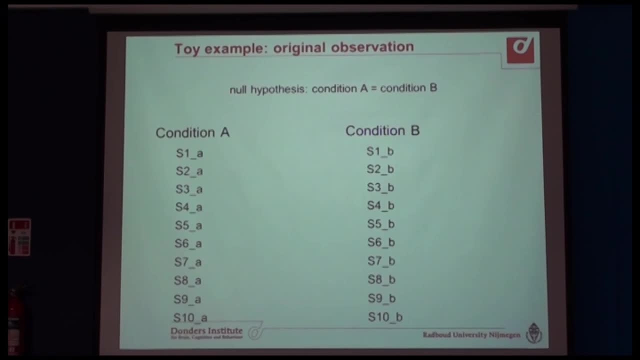 are the same. So it means that under the null hypothesis I can shuffle the data over the two conditions. And of course this shuffling where possible we will do it pairwise. So if we have observed 10 subjects, each subject in two conditions, we're only going to shuffle. 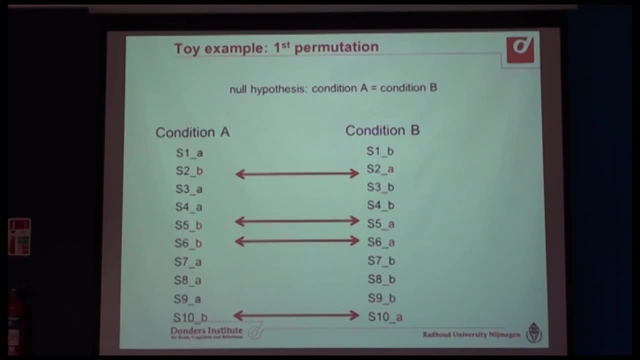 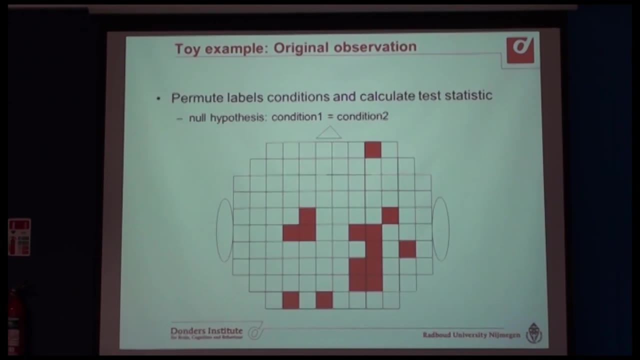 the data within the subject. so we've got, basically we're going to do a sort of a paired t-test, So it's a kind of a pair shuffling Or paired shuffling, Um, And that's something that we can repeat many times. 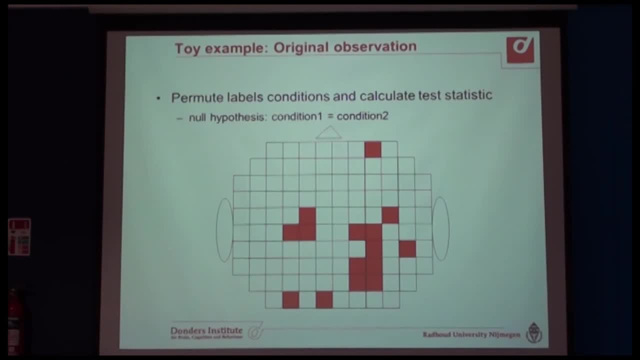 Um. And then what we have is: we can look at the spatial topography of the effect Um. So this is the original assignment. what we would, for example, observe is that there's a group of connected channels Here. the channels are indicated schematically, but we, you, can't specify the neighborhood. 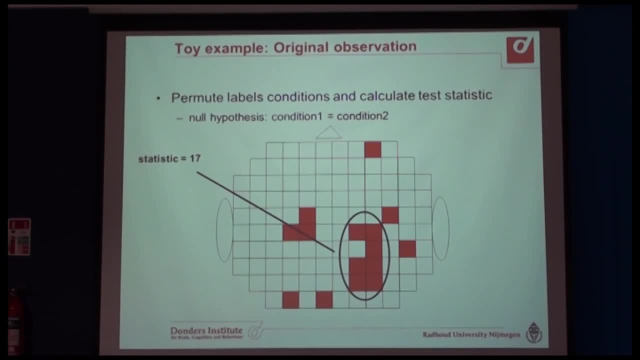 structure, So you can specify which channels you consider to be connected. Uh, you consider to be neighbors of each other, And what we'd have is all these channels are exceeding the threshold. So then, for these channels, I would look at the T-value, I would 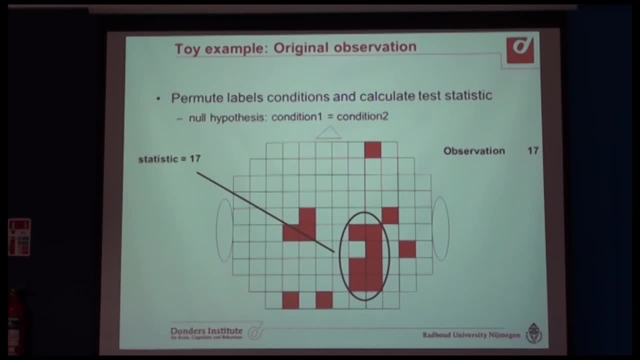 sum the T-value and I would put that in my table as an observation. Then I shuffle Again, take the largest cluster, I put it in the table, And that is something that I do multiple times. So that's basically the idea that we form the distribution of the maximum statistic. 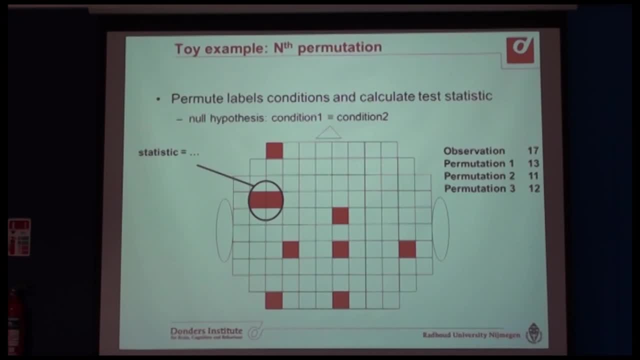 And there's quite a lot of choices that you can make, Like one of the choices that we already addressed is like: how many permutations should you make? But you can also make choices such as like: how do I compute the aggregated confidence by summing over the cluster? So 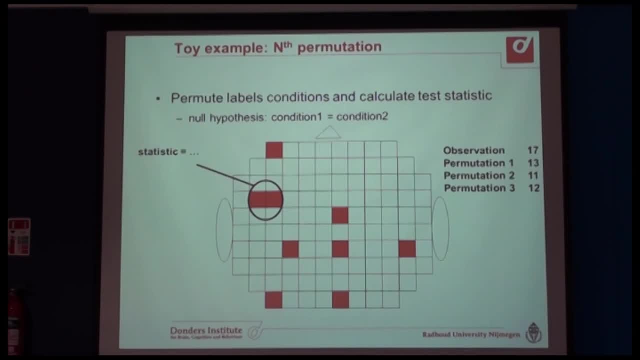 you can take the. what we normally do is we take the sum of the T-values over the cluster. You can also take the mean. You can also take the maximum value within the cluster. So basically there's a whole bunch of choices. They will affect the statistical sensitivity, but they do not affect the validity. 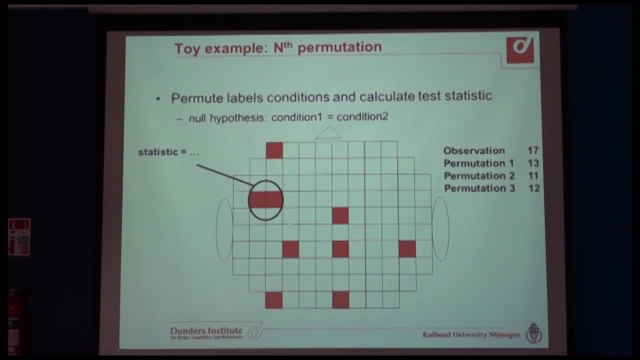 of the statistical test. Because that's all. those are all choices that you make within this black box. AUDIENCE MEMBER 6. AUDIENCE MEMBER 7. AUDIENCE MEMBER 8. AUDIENCE MEMBER 9. AUDIENCE MEMBER 10. AUDIENCE MEMBER 11. 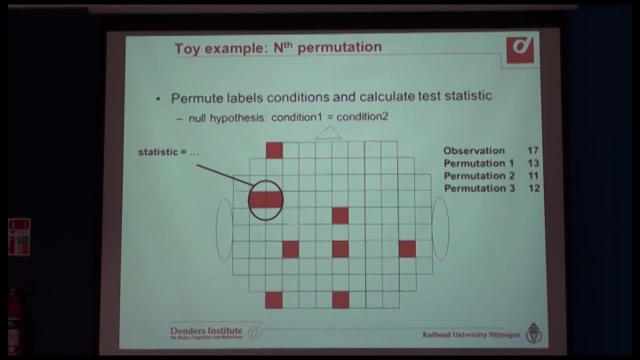 AUDIENCE MEMBER 12. AUDIENCE MEMBER 13. AUDIENCE MEMBER 14. AUDIENCE MEMBER 14. AUDIENCE MEMBER 15. AUDIENCE MEMBER 16. AUDIENCE MEMBER 17. AUDIENCE MEMBER 18. AUDIENCE MEMBER 21. AUDIENCE MEMBER 22. AUDIENCE MEMBER 23. 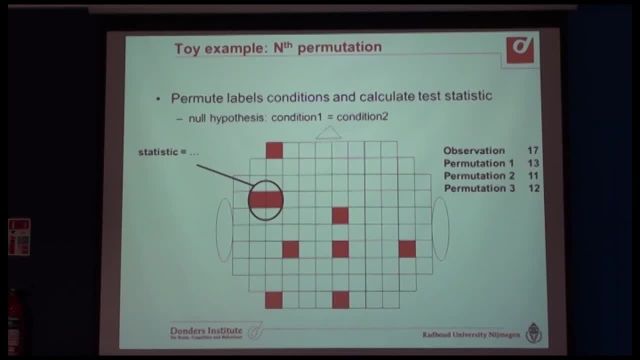 AUDIENCE MEMBER 24. AUDIENCE MEMBER 25. AUDIENCE MEMBER 26. AUDIENCE MEMBER 27. AUDIENCE MEMBER 28. AUDIENCE MEMBER 29. AUDIENCE MEMBER 31. AUDIENCE MEMBER 32. AUDIENCE MEMBER 33. AUDIENCE MEMBER 34. AUDIENCE MEMBER 35. 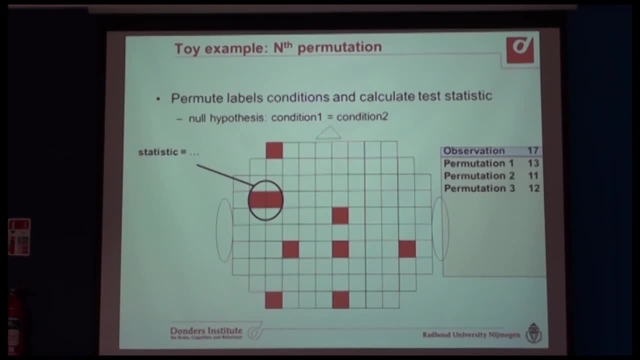 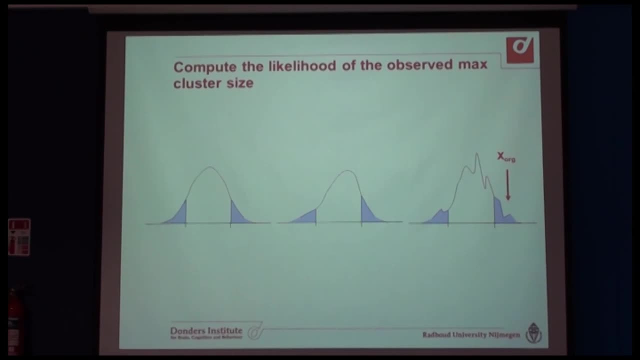 AUDIENCE MEMBER 36. AUDIENCE MEMBER 37. AUDIENCE MEMBER 38. AUDIENCE MEMBER 39. AUDIENCE MEMBER 41. AUDIENCE MEMBER 42. AUDIENCE MEMBER 42. AUDIENCE MEMBER 43. AUDIENCE MEMBER 44. AUDIENCE MEMBER 45. AUDIENCE MEMBER 46. 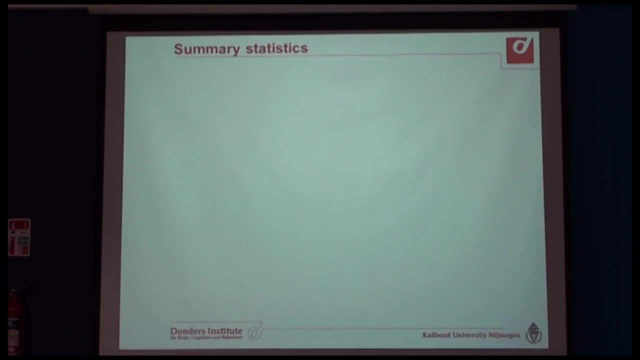 AUDIENCE MEMBER 49. AUDIENCE MEMBER 51. AUDIENCE MEMBER 52. AUDIENCE MEMBER 52. To summarize what we have is we can do parametric statistical models for many channel time frequency points where we compute the probability given a null hypothesis, where we are formally doing. 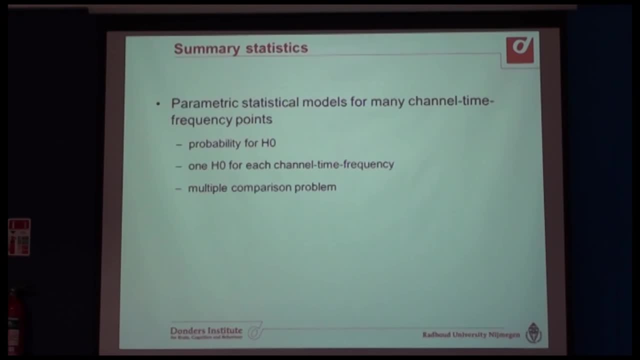 one null hypothesis for each channel time frequency point, giving a massive multiple comparison. problem With using a non-parametric approach. what we have is we use randomization or permutation. Randomization is just a subset of all possible randomization, but usually we do a permutation. 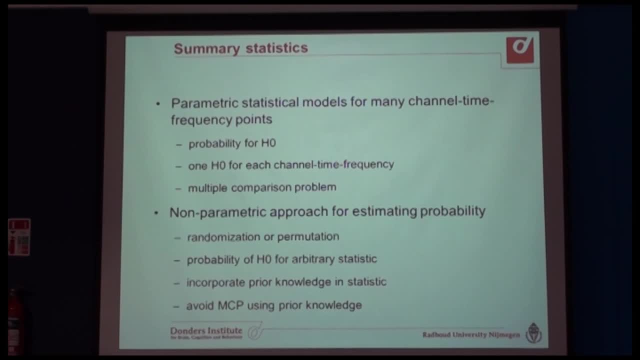 and then from all possible permutation we're taking a subset to keep the computation tractable. The probability of the null hypothesis can be computed given an arbitrary statistic. that allows us to incorporate prior knowledge into this statistic and it also allows us to avoid the multiple comparison problem using this prior knowledge. 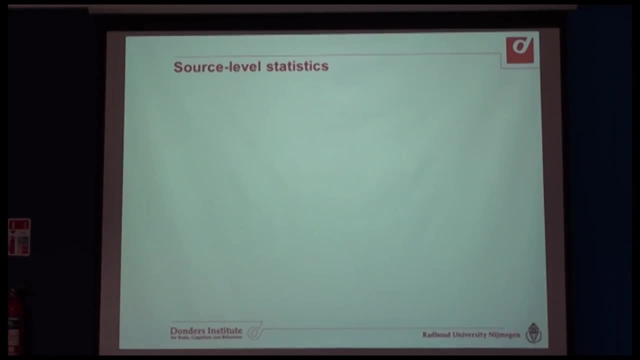 Okay, Okay, Okay. so this is so far I've been explaining everything for the channel level, but the same thing holds for the source level and I think it is valuable. it is important that with MEG data, that we go to the source level, like that's the whole point of having a whole 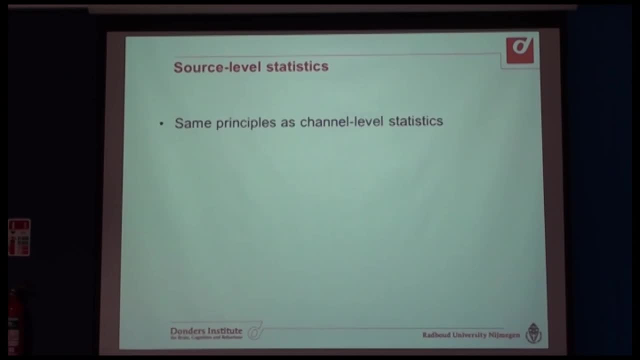 channel, a whole head, many channel MEG system. So for source level, the same principles apply and the idea is that for beamforming, for example, that would swap the data between the conditions. However, if we do that, if we just swap the data at the channel level and then we compute, 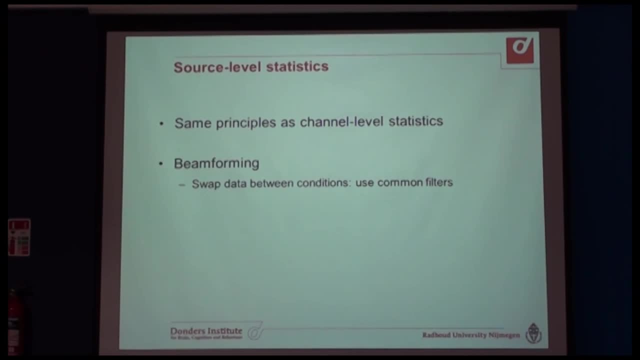 spatial filters and we compute the beamformer distribution of power all in this black box. that's computationally. it's very expensive because it's like a beamformer. analysis will take a second or a few seconds, maybe five seconds, which means that if you have to do 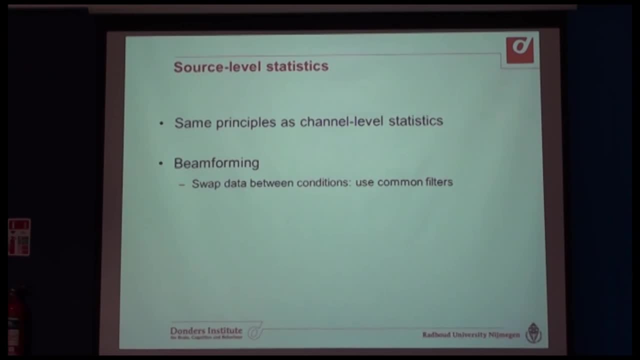 a thousand randomizations, you're looking at some serious computational time. So that's why we can consider actually how this beamformer formulation works and that's where the common filters come in. So let me first explain a little bit how we organize the data. 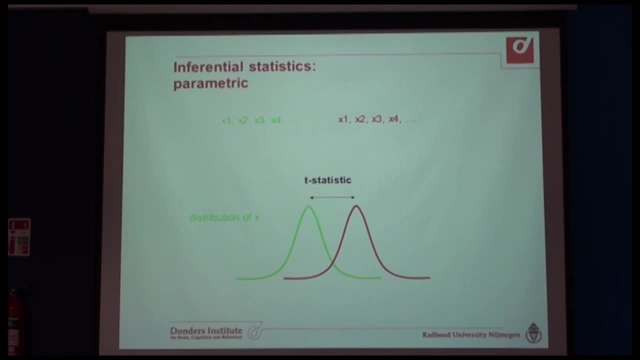 So what we have is: we have data, we observe it in two conditions. and if we're considering the data at the source level, then what we have is, for example, a three-dimensional volume, and this three-dimensional volume has dimensions along the x and the y and the 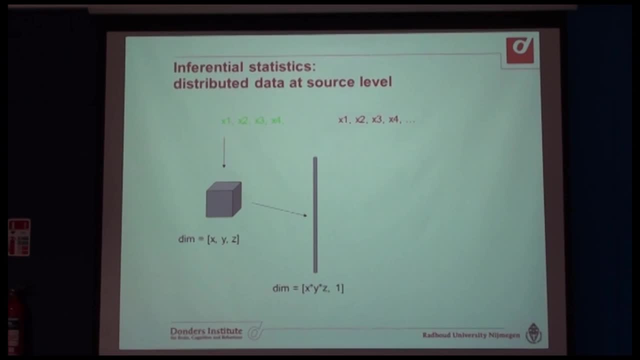 z direction, and what we can do is we can reshape this into one very long vector, and that is how it's internally done in these functions. Each of the elements of this vector is basically is one voxel. So what I then can do is I can plot the data into two conditions like this: so I have my 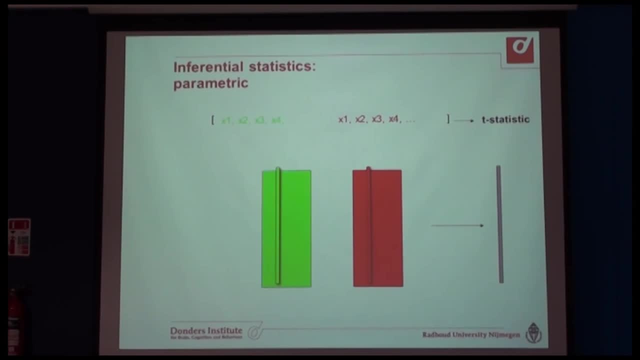 observation in one condition, I have my observation in the other condition. this is one condition, this is another condition and given these volumes in each of the conditions, I can compute a t volume, like I can compute a statistical parametric map. and of course, the idea is: 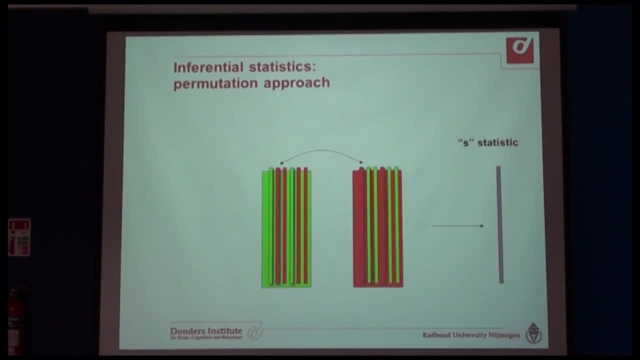 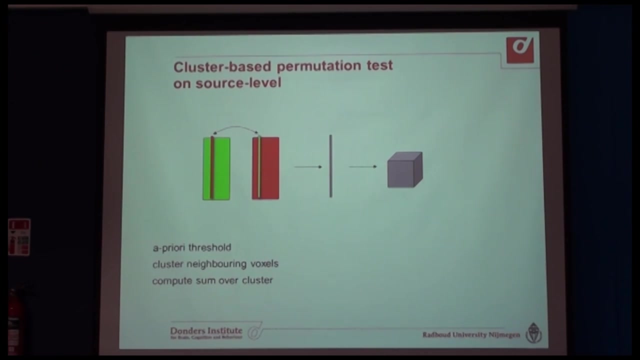 that we out-shuffle the data between the two conditions, and that's why we have a three-dimensional volume Again. I would do that many times and every time I would compute this t volume. So, given this volume of t values, or giving like, which I can again reshape into this: 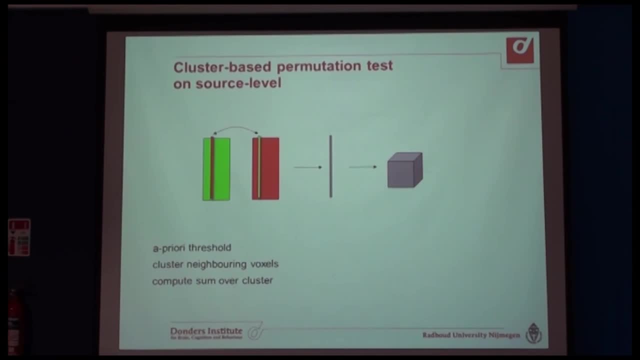 whole-brain grid representation. I can set an upward threshold and I can cluster neighboring voxels and again I can compute the sum over the clusters. So if we now return to beamforming Under the null hypothesis, I'm claiming that the data comes from the same distribution. 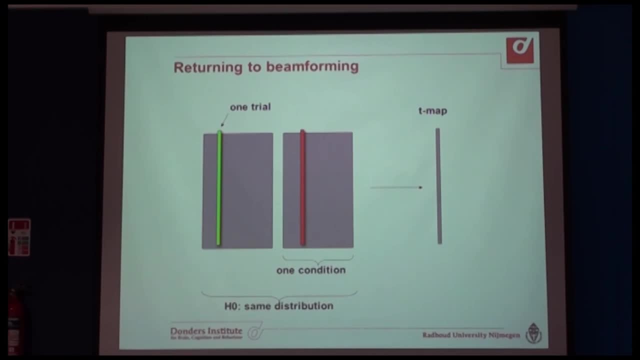 that the data is the same. So, although this is one condition under the null hypothesis, the data in both conditions is coming from the same distribution. So that means that, rather than computing a spatial filter for one under the null hypothesis, the best spatial filter that I would be able to compute would be the one in which I use. 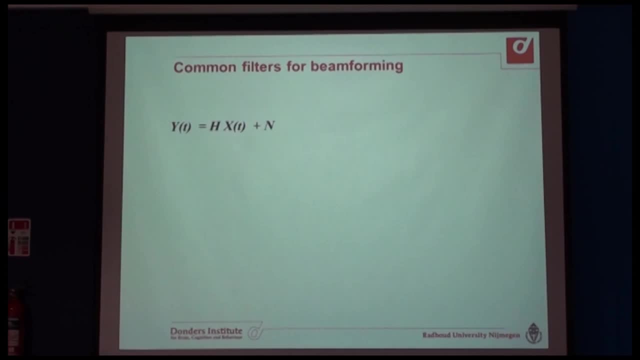 both data sets. So let's look at the mathematics here. So yesterday Joanna showed that we have this forward model. so the channel-level data is the lead field, times the sources plus noise, and what we do is we compute the estimated source, which is a spatial filter, times the channel-level data, where the spatial filter 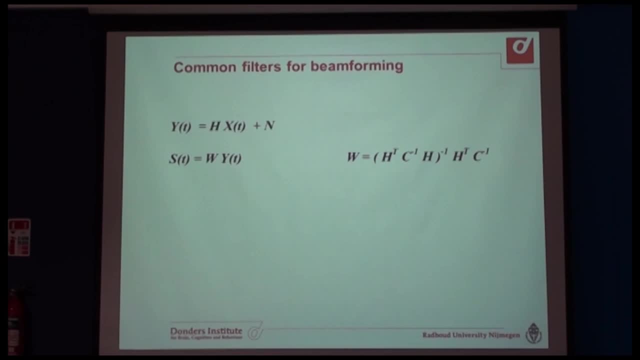 is computed like this, and the spatial filter has the lead field in it and has the channel covariance matrix in it. right, I might be using slightly different letters than Joanna used yesterday, but like the structure of the equation should be clear for you. 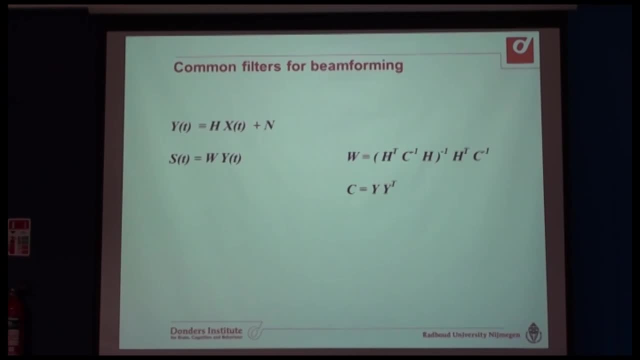 Okay, so what we have is we have the covariance matrix, and the covariance matrix is basically the data times, the data transposed divided by the number of data points. What we also have is the power, the source-level power, and the source-level power is basically: 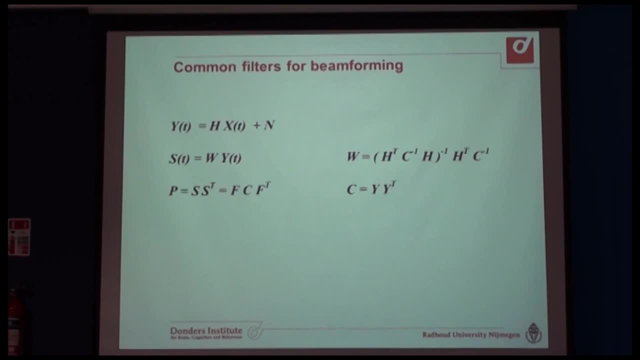 it's the source-level time series times the source-level time series transposed. it's the variance of the source And if I just, rather than taking these, I can also take these. actually, just, I'm inconsistent here myself because this should have been a W. Sorry about that. 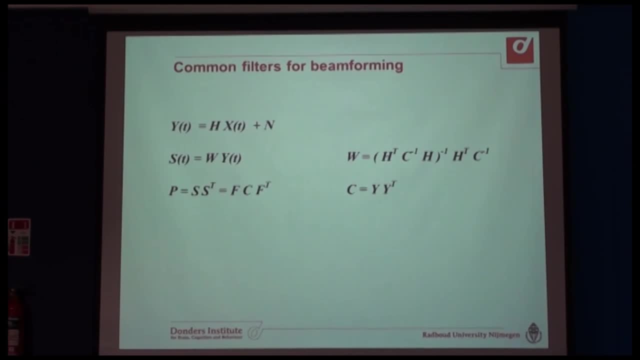 So, but what I have is I have W times Y, times Y transposed, times W transposed, because what I'm doing is I'm using this equation to fill in here. Okay, So that means that if I consider the covariance matrix, well, the covariance matrix is basically: 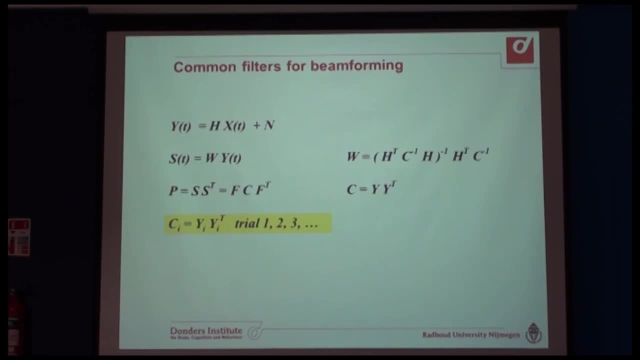 it's the sum of the covariance matrices or the average of the covariance matrix over all trials. So the covariance matrix, the average covariance matrix is basically, is this one. Of course I can try to compute single-trial beamformers, but my covariance matrix, my 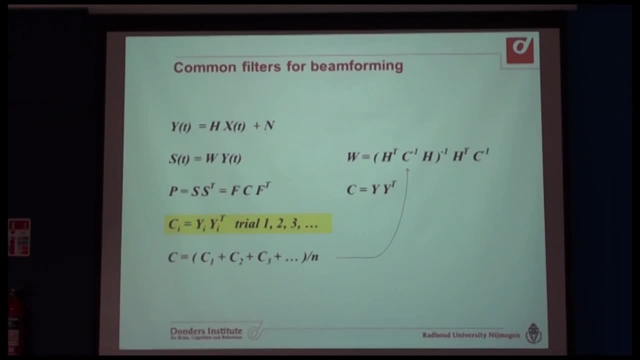 estimate of my covariance is very poor, so single-trial beamformers are extremely noisy. So that's why we always compute beamformers on the averaged covariance matrix or on the average cross-pectal density matrix. So but if so, here and here you see the averaging over all the trials. 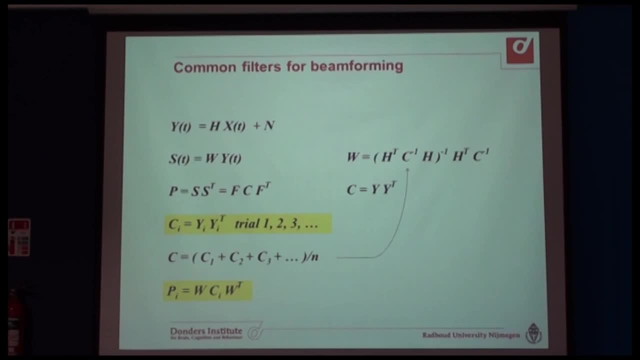 But the nice thing is that if I take the average cross-pectal density or covariance matrix in computing the filters, I can very easily compute single-trial power by, rather than here taking the power for the average cross-pectal density matrix. 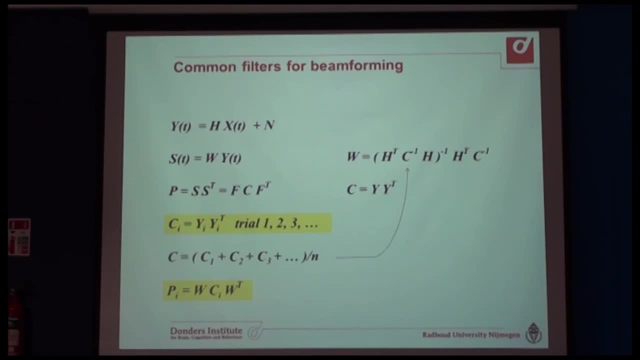 I just multiply that. Okay, I multiply my filters with a single-trial covariance matrix. So what I'm doing is I'm splitting the problem into estimating the filters and estimating the power, And that means that, given the null hypothesis that the data's coming from the same distribution, 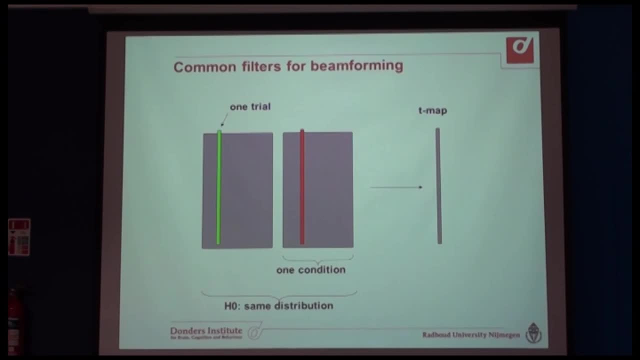 I have. the best spatial filter that I can compute is the one where I've averaged all of the data covariance into one covariance matrix and I'm given the covariance matrix in the same distribution. So, in other words, I don't ever have to go back and look at the returns of any returns. 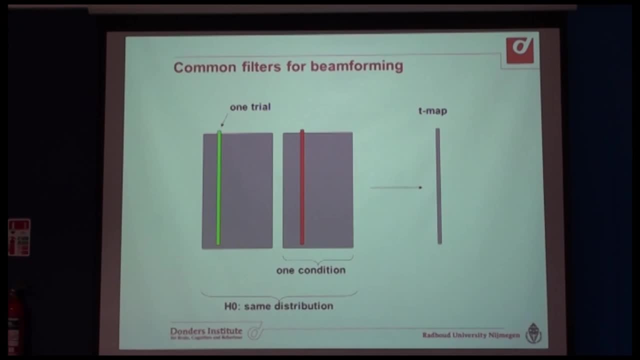 from the previous Australia, but I'll be able to compute them from there. So, in order to do that, and then, of course, in this case, in each individual trial, I can compute the power in each individual trial, And if I can compute the power in each individual trial, and that's done just by a simple multiplication, 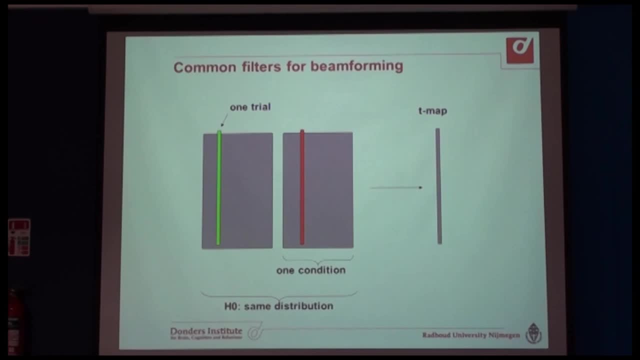 I can very easily get start shuffling these trials. Yep: Male Speaker. 3. Male Speaker. 4. Male Speaker. 5. Male Speaker, 6. So my single trial power estimates will still be relatively noisy, but if I let's go back here. so what I'm doing here? in the computation of the filter I'm taking the inverse of the covariance matrix. 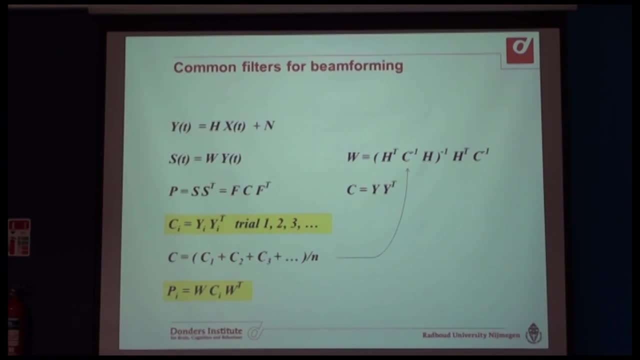 Taking the inverse of a very noisy covariance matrix is going to give an extremely unstable inverse. So that means that the spatial filter that I can compute, like the computation of the spatial filter, is a nonlinear operation. The spatial filter that I can compute for a single trial is going to be extremely noisy. 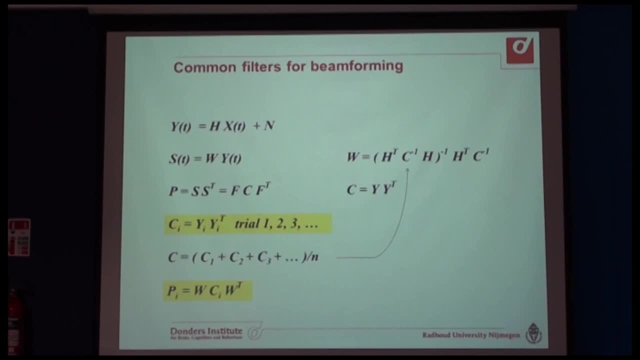 The spatial filter that I compute for all the trials together is quite a stable filter. The multiplication of the spatial filter with the single trial covariance, that's a linear operation. So the average of my single trial power given a common filter is the same as the spatially filtered average data. 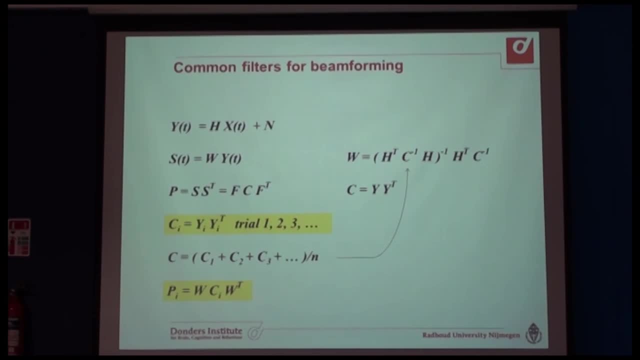 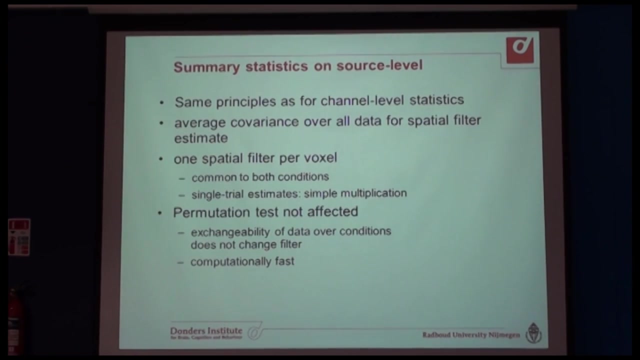 Because that's a linear operation, But it's the non-linear operation of the computation of the spatial filter that is sensitive to this noise, to this poor estimate of the noise. Yeah, Okay, so with source level statistics, basically we're using the same principles as for channel level statistics. 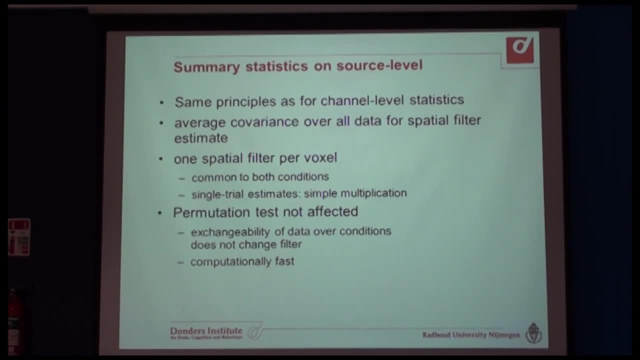 We start- and basically it's a two-step approach and that's also what you've seen yesterday In the hands-on. we start with an average covariance over all the data to get the spatial filter. We have one spatial filter for each of the voxels. 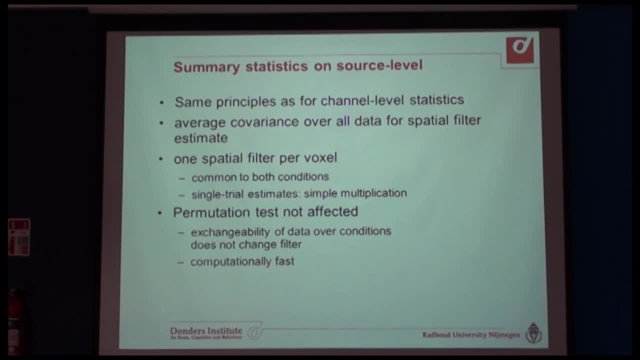 And under the null hypothesis that spatial filter is not going to be different. So best to compute one spatial filter And that allows us to do single trial estimates by just a simple multiplication. So that means that we can compute single trial power quite robustly for a thousand. 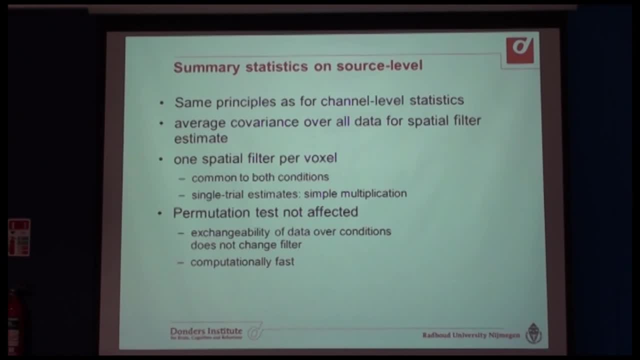 Different randomizations of the data And it's also fast, Like that's only a few, like a minute or so. The permutation test, however, is not affected, Because what we assume is that we assume exchangeability of the data over the conditions. 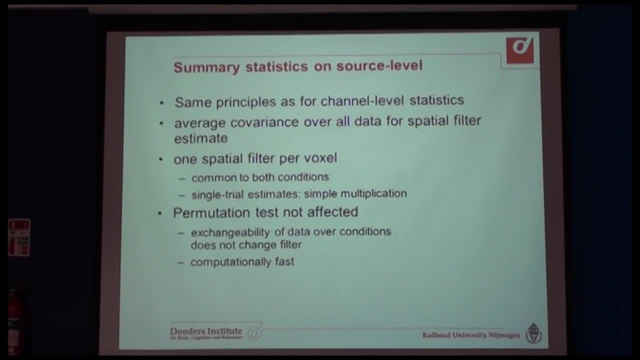 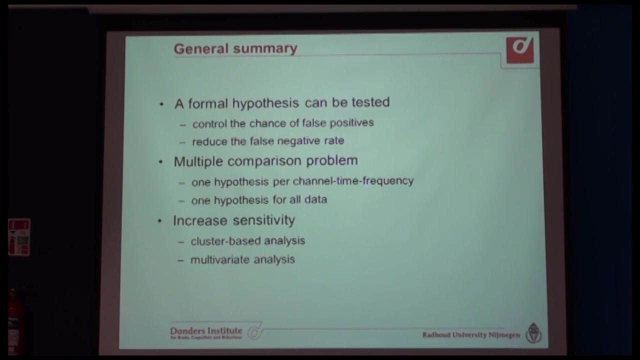 But if we exchange the data over the conditions, the spatial filter doesn't change, Which means that it's perfectly fine to compute the spatial filter in advance And, yeah, so it's computationally fast. So, to wrap up, what I've shown is that we have a method for testing a formal hypothesis. 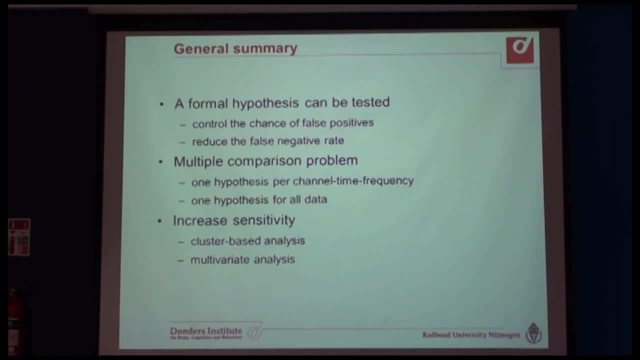 Which allows us to control the chance of false alarms, And that's important because, although we take the risk, if we're publishing a paper, that's basically that the finding cannot be reproduced by others. We don't want to publish too many papers that cannot be reproduced, right? 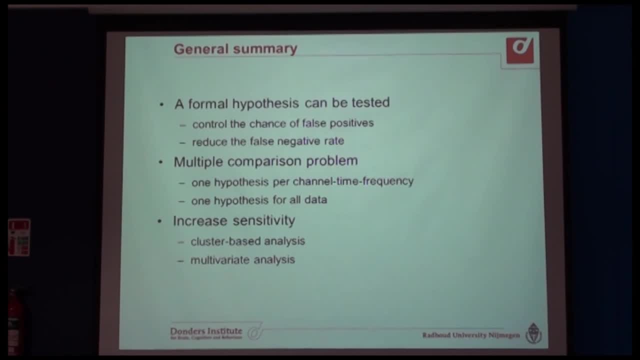 So we have to control the chance of us making false claims, But at the same time we also don't want to be overly conservative, Like if you're using a Bonferroni correction at the channel level, then you'll never publish a paper. 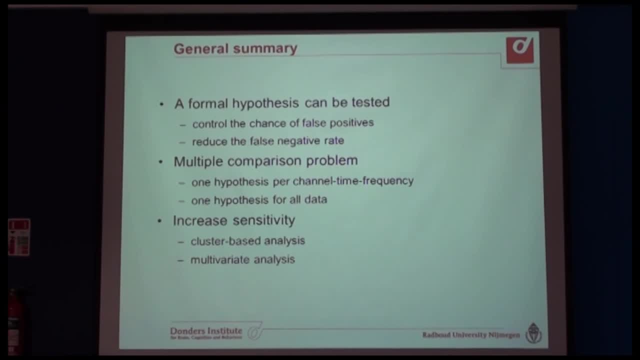 That's also not good. So we want to control the false alarm. We want to have not too many false positives, but you also don't constantly want to have false negatives, And that's why the increase of the sensitivity is such an important aspect. 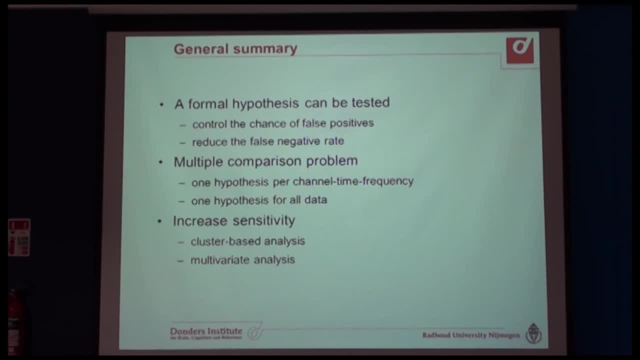 The multiple comparison problem mainly comes about by having one hypothesis per channel, time, frequency point or one hypothesis per voxel. And the way that the cluster-based randomization test circumvents the multiple comparison problem is that it replaces multiple comparisons by a single one, So by taking the value of the maximum cluster. 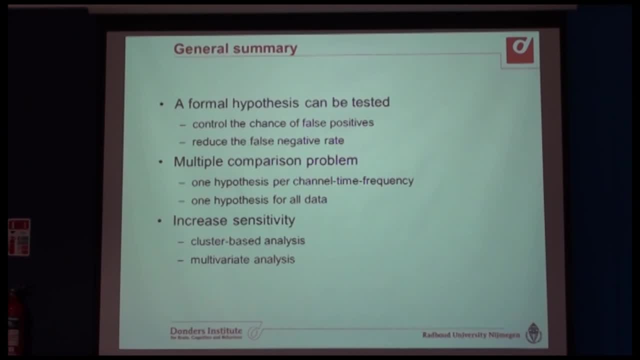 And that is a That's a valid approach, because if we reject the null hypothesis, then we know that the alternative hypothesis holds, which means that the data is different And we increase the sensitivity by not taking only the maximum statistic, but by taking the sum of the values within the largest cluster. 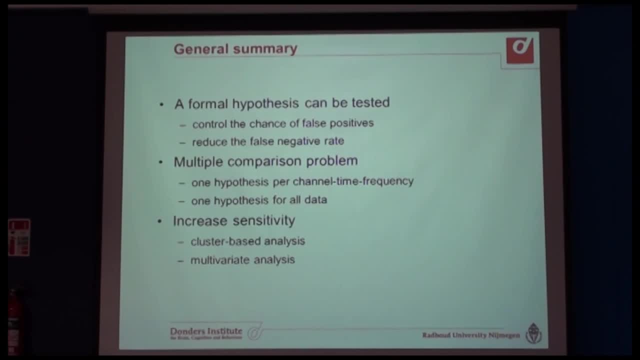 And, as such, this is a- Although we start with a massive univariate statistical map, we are combining values over multiple voxels, So it is a sort of a multivariate analysis that we're doing. inside this black box, There's- I think there's, two more important aspects to mention. 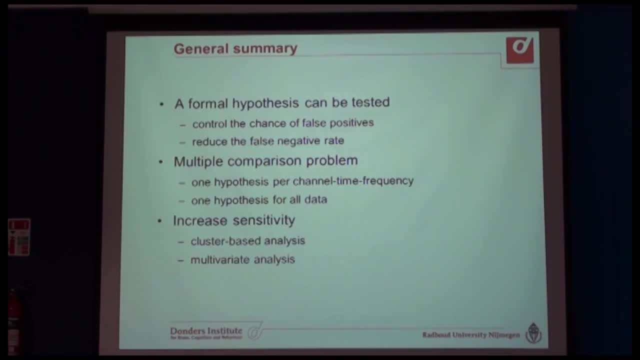 And the first is that we're making an assumption about the data being exchangeable under the null hypothesis, Which means that if we reject the null hypothesis, we can firmly conclude that the data is not exchangeable. It does not necessarily instruct us what the feature in the data is. 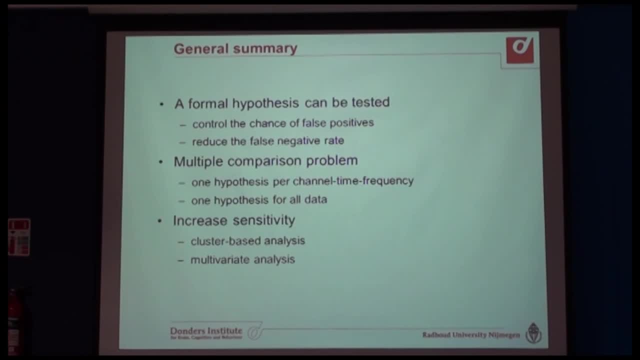 It does not instruct us what the feature in the data is. It does not instruct us what the feature in the data is. So a lot of people have the tendency to say, well, I have a significant cluster. Well, it's not the cluster that is significant. 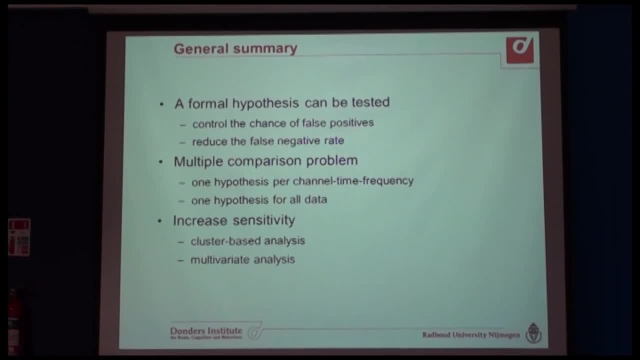 You have significant effect, allowing you to reject the null hypothesis. There is a difference in the data and the difference is expressed in the cluster, But it's not only the cluster where this difference happens, And that's especially obvious if you consider channel-level data. 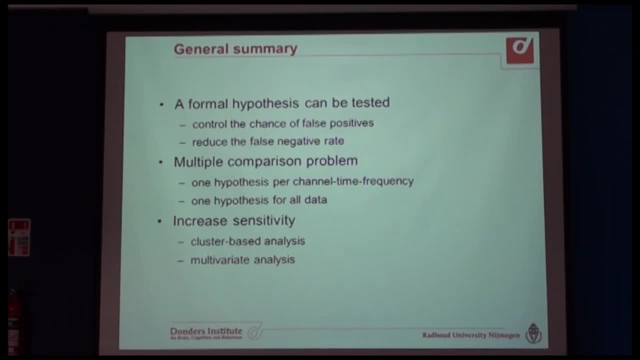 So of course you will have a source somewhere in the brain Projected towards the scalp And on the scalp some channels will show a large effect. So if you threshold the scalp-level data, then on those channels you're going to find a cluster. 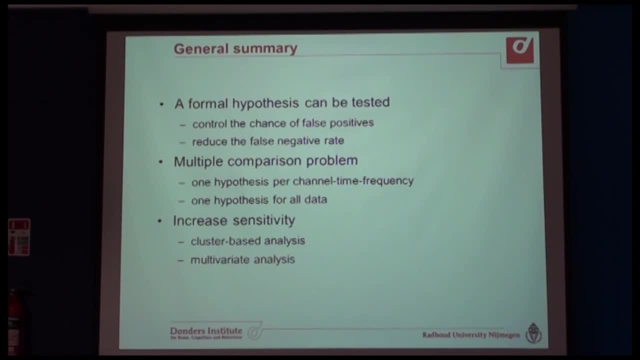 And on the basis of that cluster, you're going to reject the null hypothesis that the data is exchangeable. But if you find an effect on a few channels, well you know that the source is projecting to all channels. It's just projecting more strongly to some channels and more weakly to other channels. 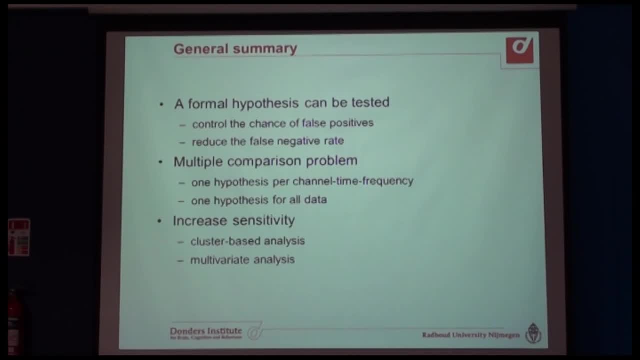 So you should not interpret that, You should not interpret that cluster as having the significant effect. The significant effect is actually in the brain, It's not on the channels. And, in principle, if you had recorded more data, if you had recorded more trials, then the cluster would have gotten larger. 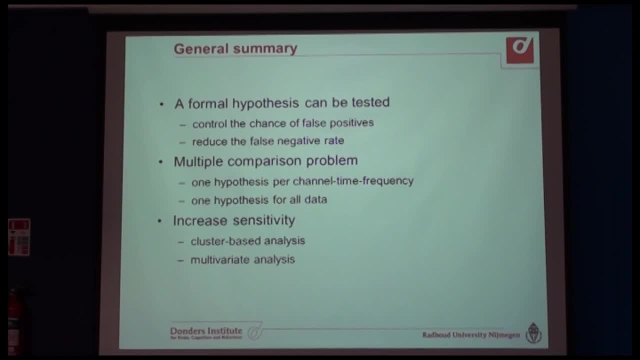 Like you, would have been able to show on more channels that there would be an effect. So this thresholding, this clustering, you should not take it as an interpretation of what the difference in the data is. So the decision that you make in rejecting the null hypothesis is still 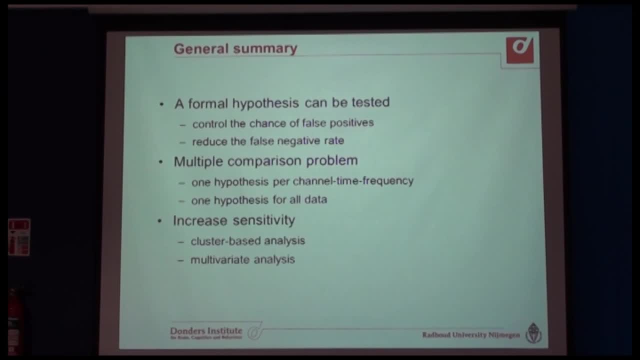 relatively independent from you interpreting the difference in the data, And that's an important step. Like the interpretation of the findings, is different from the statistics. Statistics is only a tool to help you make an informed decision, But statistics is not a tool for you interpreting the data. 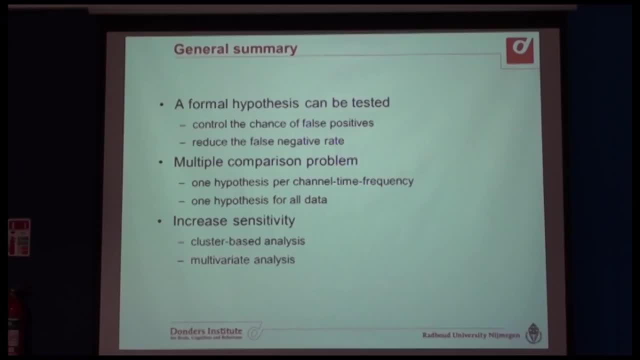 The second point to make is that I've always been talking about exchanging data between two conditions, And you already came up with the idea Like. so How about like a more ANOVA type of model with multiple factors or a repeated measures ANOVA? 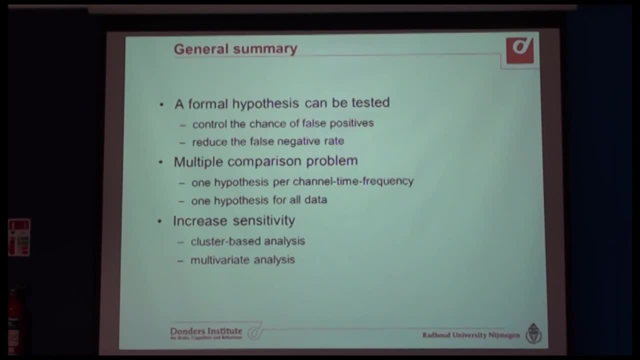 What I'm saying is What I'm stating is that we have a hypothesis that is not dependent on the parameter in the data Once we start doing ANOVAs. actually, we are assuming a model of the data, We are assuming parameters of the data. 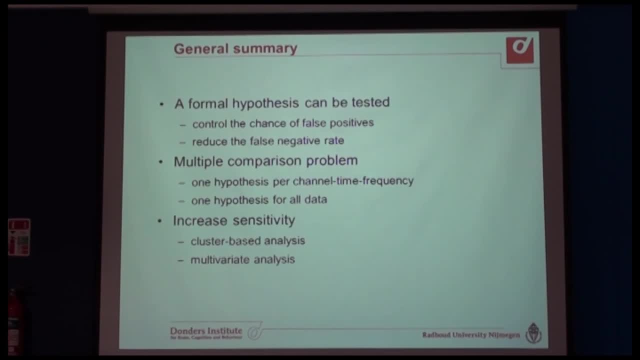 We're assuming that the data can be described using the mean value and using variances. So that means that the In general, In general, the model of an ANOVA is incompatible with a non-parametric test, Because an ANOVA is a parametric model. 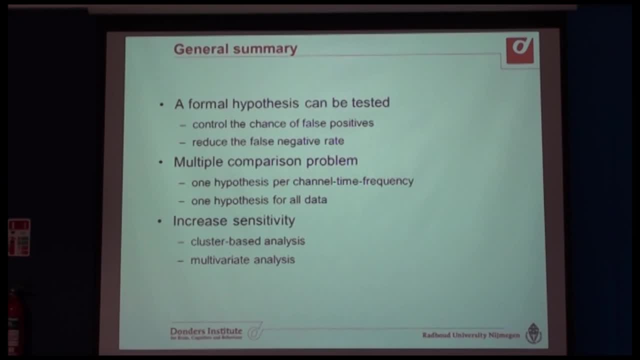 And it means that usually if you do an ANOVA you're not interested in the main effects, but you're interested in the interaction, And that interaction only applies if you assume that you have a linear model. So that means that in principle an ANOVA is incompatible with a non-parametric test such as this: 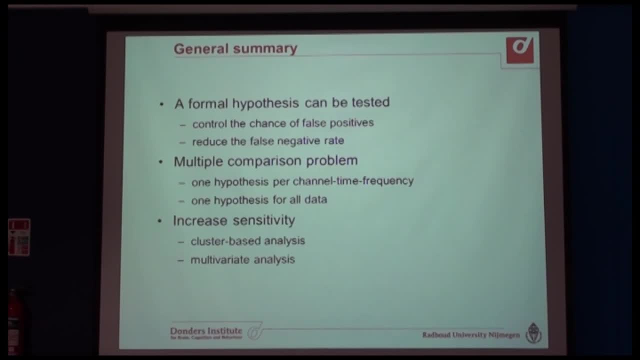 However, there's a workaround. What you can do is you can do a first-level descriptive statistical computation of your interaction effect And then, on the second level, you can test whether that interaction effect is, For example, whether the sign of that interaction effect is exchangeable. 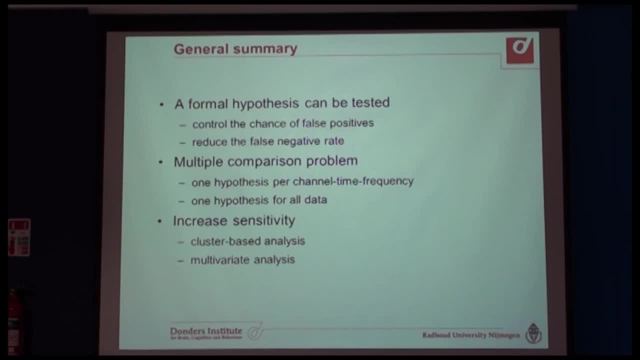 So what we often do is we do a two-tiered approach, where on the first level we compute a descriptive statistic And on the second level we do the inferential statistic, given the first-level statistic. So the first-level statistic would be the interaction. 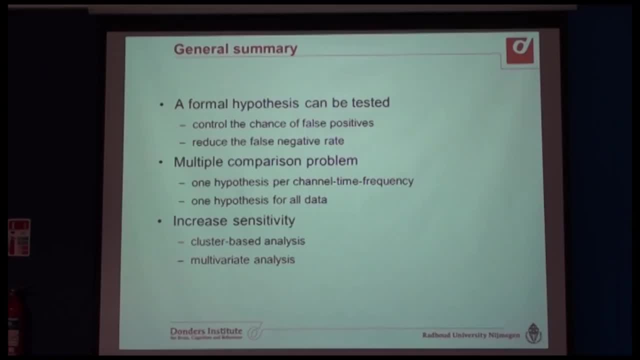 And the second-level statistic would be whether that interaction is consistently, If we flip the sign of that interaction, whether that would be the same, Because under the null hypothesis the interaction would have a random sign. It would be positive for some randomizations, negative for some others. 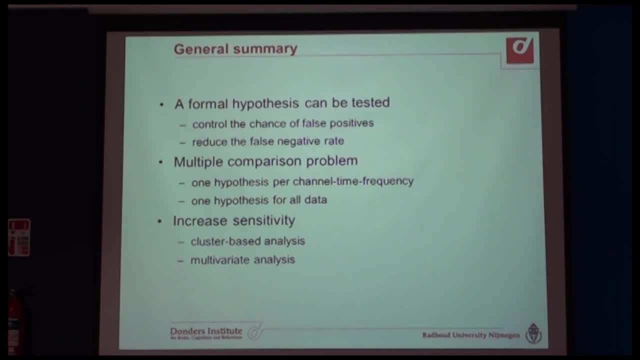 So that's basically the trick that we use to test parametric models. It's a non-parametric test, but using the If in the parametric model. if you use that in the first-level test, then you can take the first-level statistic to the second level. 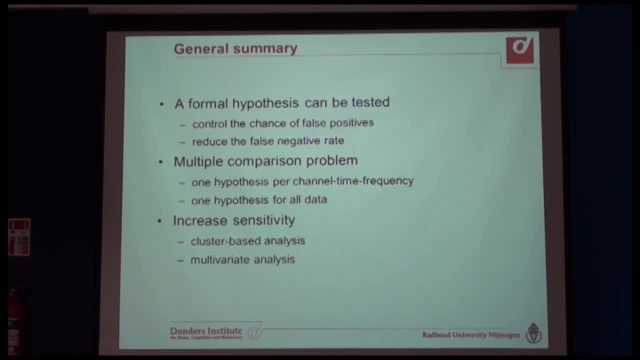 And at the second level, we do the statistical inference. Yeah, but the interpretation is invalid Because the interpretation is an interpretation about the data, not about the model that you're testing. So what we can do is we can show that the data is. 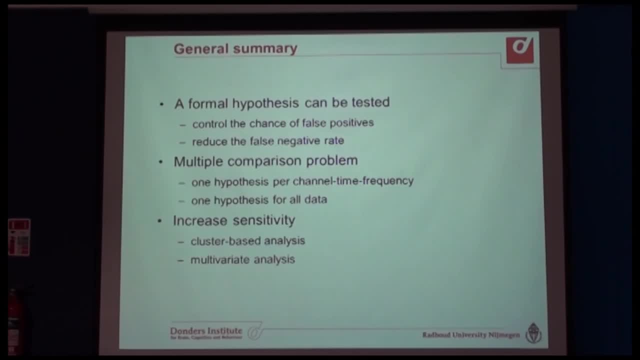 not exchangeable. but you still don't know whether there's an interaction effect. Because although you're computing the interaction effect as the statistic, it's the same as if we reject the null hypothesis on the basis of the cluster. it's not that the cluster is meaning something. there's something different in the data. 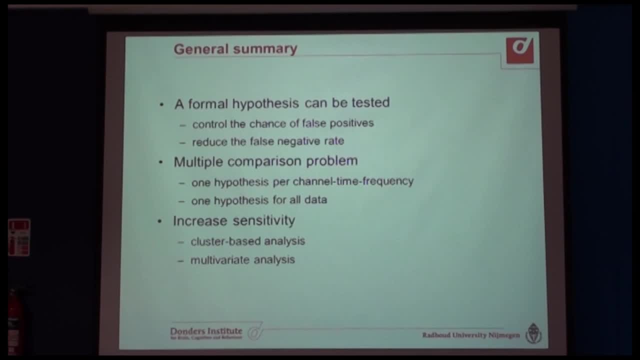 So that's why it is important to understand that the statistical procedure is rejecting the null hypothesis And the null hypothesis is not about a parameter. So the null hypothesis is not about the interaction effect. The null hypothesis is not about the mean values. The null hypothesis is about exchangeability of data. 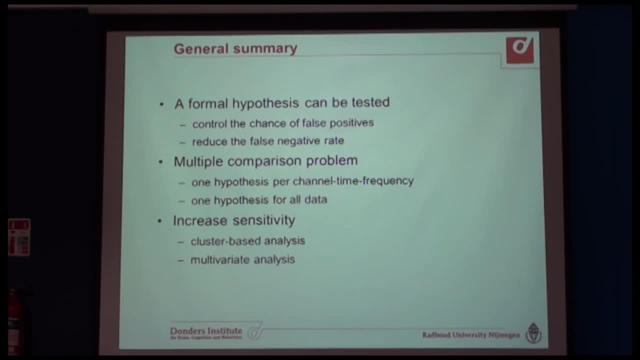 And that null hypothesis does not change. So if you compute an interaction effect, if you compute repeated measures, ANOVA, it's not going to change the null hypothesis. Which means, if you reject the null hypothesis, you still don't know anything about the interaction between the two main effects.